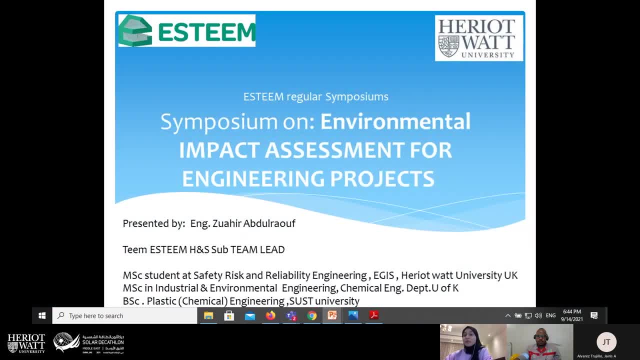 Symposium, STEAM is a solar decathlon society of Harry World University. We participate in the SDME competition held in Dubai by building a smart home to tackle problems of climate change. Our aim through Symposium is to elaborate our field of expertise and provide a learning platform. 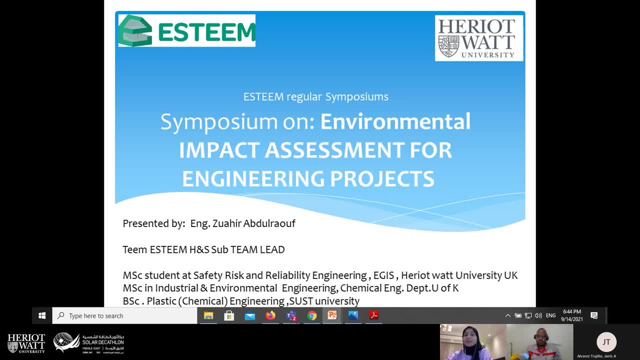 about the technologies, principles and ideologies involved with STEAM. We will be having a practical learning interactive segment at the end of today's seminar where you can ask any questions related to the topic to our guest speaker. We will be recording the seminar as well, so if you want, 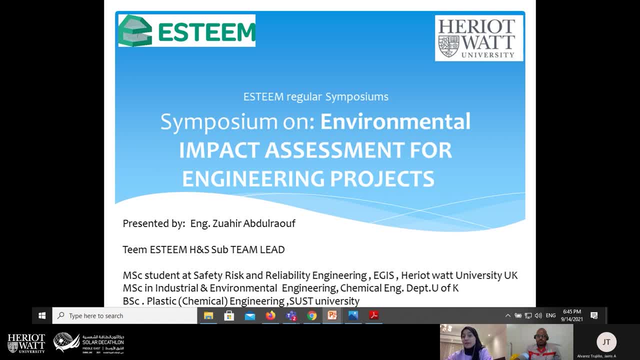 to refer to it later or show it to your friends. you can see a snippet of it on our social media platforms or ask us for the recording link via email. Also, if everyone could just type in your email ids at the chat box so we can send the certificates of participation for. 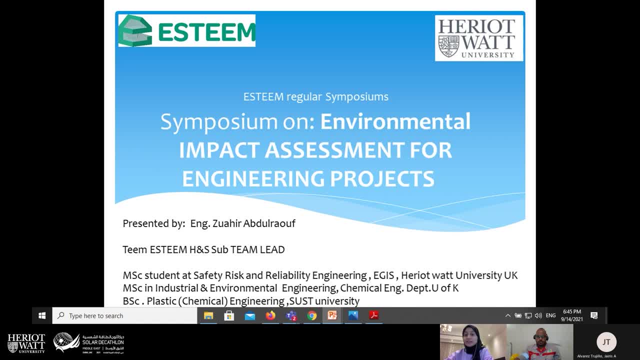 attending this educational seminar with you, which you can share on your LinkedIn, Instagram, Facebook, and if you could tag us while you do so, it will be great. So, without further ado, I'd like to welcome our guest speaker for the seminar today, Zuhair Abdul Arouf Ahmad, who will be speaking. 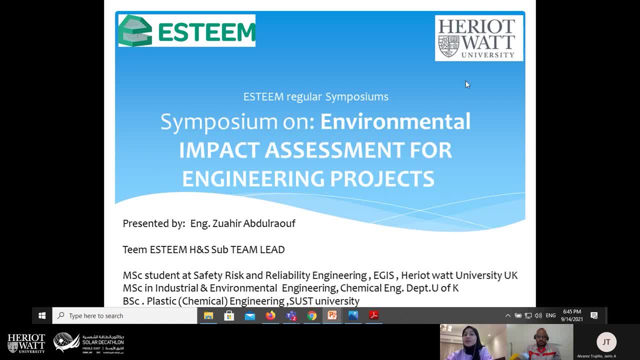 on Environmental Impact Assessment for Engineering Projects. Zuhair is studying Master of Sciences, Safety, Risk and Reliability Engineering from Harry World University and has a Master's Degree in Chemical Engineering from University of Khartoum and a Bachelor of Science in Plastic and Chemical Engineering from Sudan University of Science and Technology. Zuhair is currently 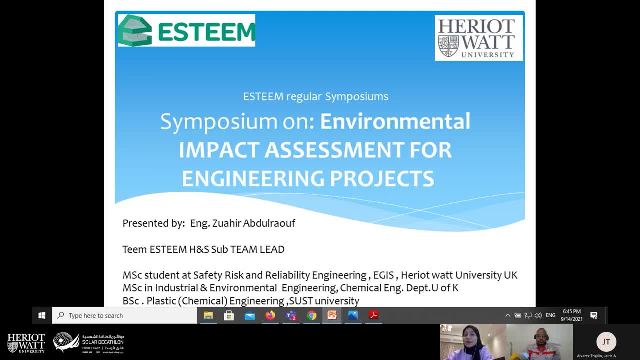 working as the Field HSE Officer for Sharif Petroleum Operating Company and has an experience of over 10 years in this field. Zuhair is also the Health and Safety Team Leader for his team. He will be covering topics like EIA Screening, Scoping, Concentration, Reporting and Removing. 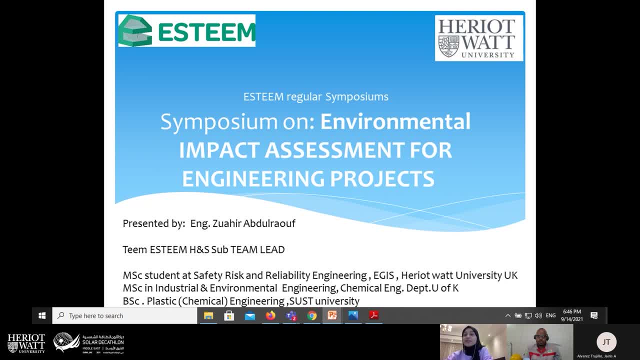 You can any questions you might have in the chat box throughout the presentation or raise your virtual hands with the MS Teams feature on your device and I'm sure Zuhair will be happy to answer them all Over to you. Zuhair, Thanks, Mideha, and welcome all. It's my pleasure to present today a topic on Environmental Impact. 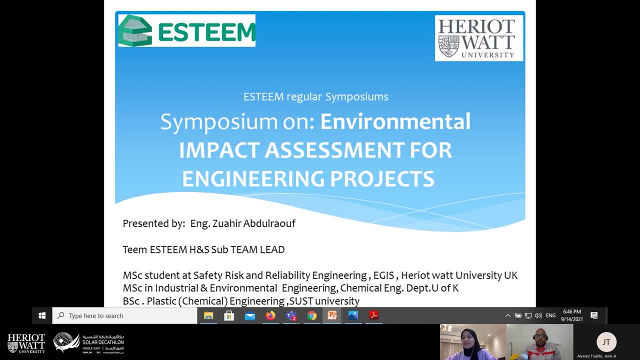 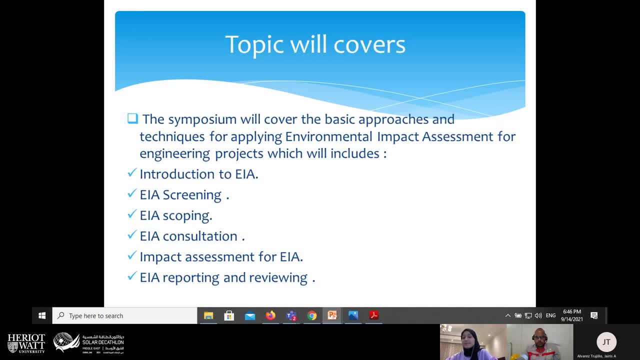 Assessment for Engineering Projects. We will talk about overview of Environmental Impact Assessment. We will talk about introduction to EIA, EIA screening, then the third step will be EIA Scoping, EIA Consultation and Impact Assessment for EIA. and then, at the final, we will talk about EIA. 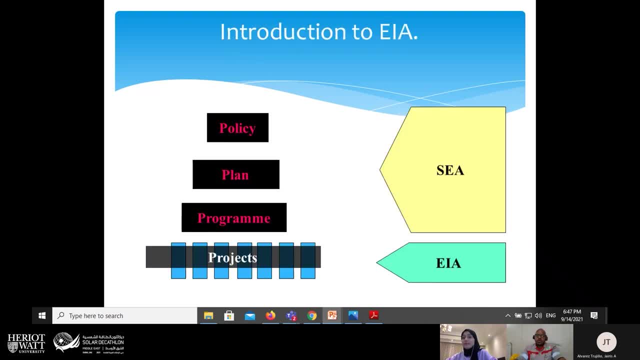 Reporting and Reviewing. As you know, all the strategic planning and state planning as general content are starting from the policy, then the state or the government has a plans and then also have some programs. Under all this umbrella the projects came. So there is a two kinds. 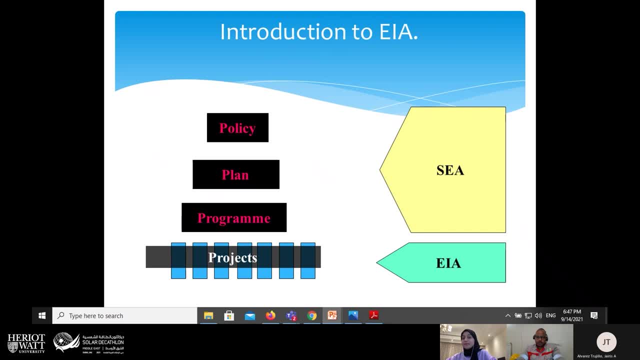 of environmental assessment for those criteria. We have SEIA, which strategic environmental impact analysis, and we have also EIA Scoping and Reviewing, which is really a strategic environmental impact analysis, and we have also environmental impact assessment, EIA. So the EIA focus on the project, but the SEA focus on the. 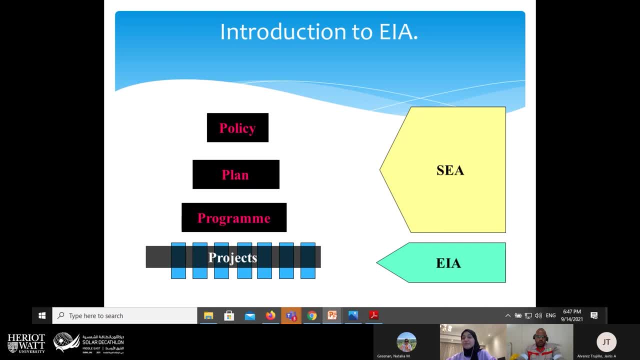 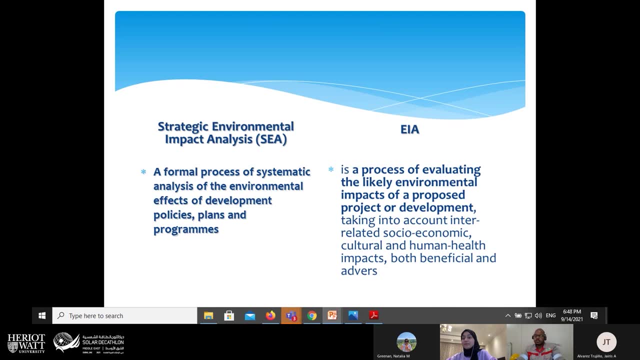 policy, plans and programs. Today we will talk about the EIA, which is a process of evaluating the likely environmental impact of a proposed project or development, while the SEA, or the SEA it, is focusing on the- as we talked before, on the plan itself and policies and programs. So 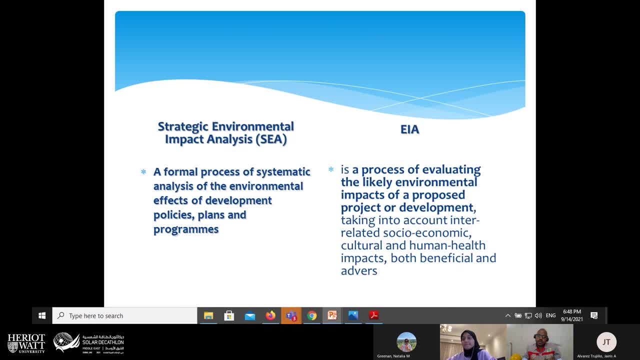 the government usually used SEA to identify or to take the decisions on either we could go for this plan or this plan. but EIA used usually to identify either we can go to this project or that project, or whether it is a useful tool to identify the how the deep we can go or inside. 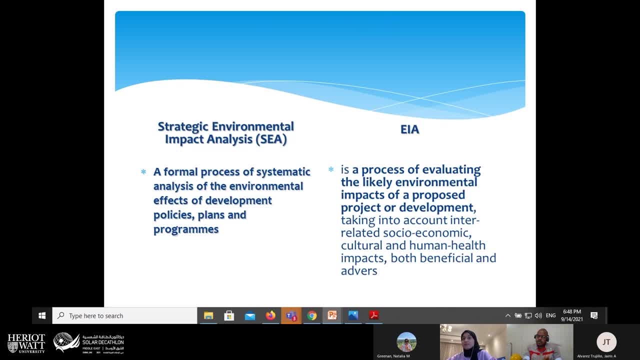 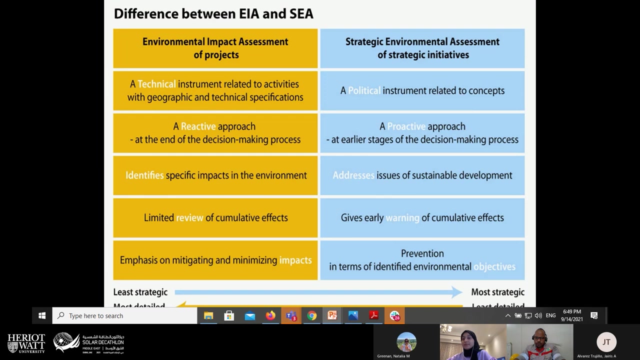 these projects or we could not take at all that this project. So it is a process, as we said, evaluating, of evaluating the likely of environmental impact of a proposed Difference between SEA and EIA. it is reflected in this schedule. we have the EIA focusing usually in. it is a reactive approach, usually used at the end of 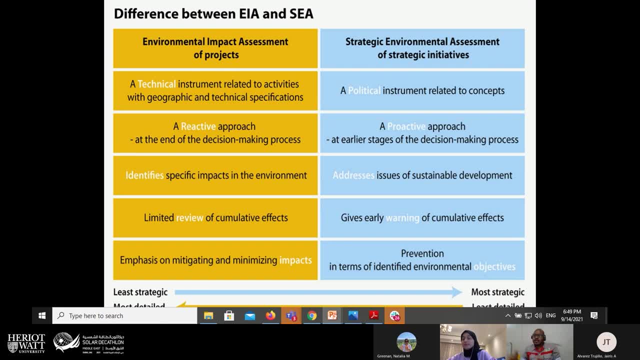 decision making. as we said, the SEA, rather than that focus on it, is a proactive approach and it is at the earlier stage of the decision making because at the stage of plans and programs we could use SEA to identify the risk and identify the impact and then decide about the better plan we 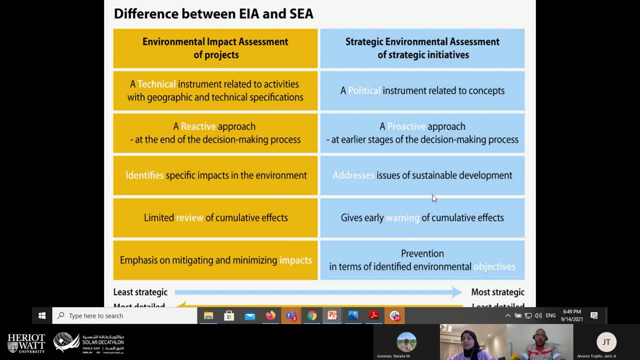 could go with. So, as introduction to EIA, we need to talk about the EIA purposes. The aim of environmental impact assessment is to identify the risk and then decide about the better plan we could go with. So, as introduction to EIA, we need to talk about the EIA purposes. 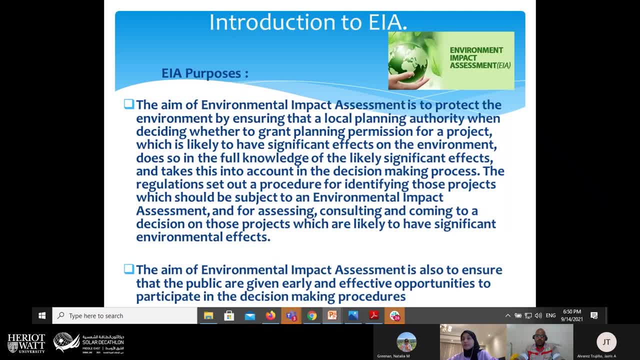 The aim of environmental impact assessment is to identify the risk and then decide about the better plan we could go with. So, as introduction to EIA, we need to talk about the EIA purposes. The aim of environmental impact assessment is to protect the environment by ensuring that a local planning authority 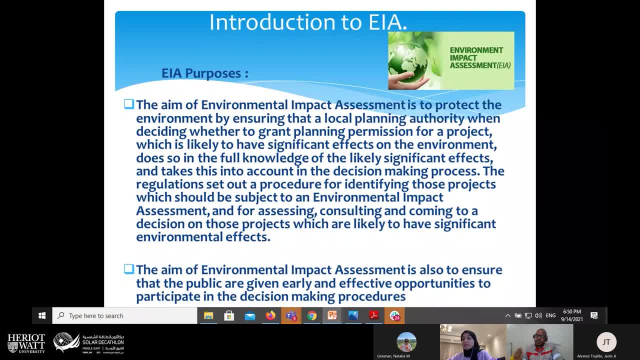 have good information to take the decision. So the EIA help the local planning authorities to take the right decision while comparing the different projects and while evaluating the project itself, so we could use it as a very useful tool to have a good decision, as we talked before. 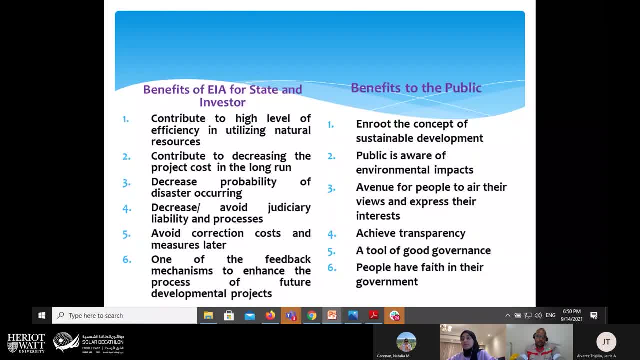 So we need to know about the benefit of EIA for the state and the benefit to the public, To the state, an investor, it is had. efficiency in utilizing natural resources Also could decrease the project cost in the long run run. because we are focusing, we are dealing proactively with the impact, so we could 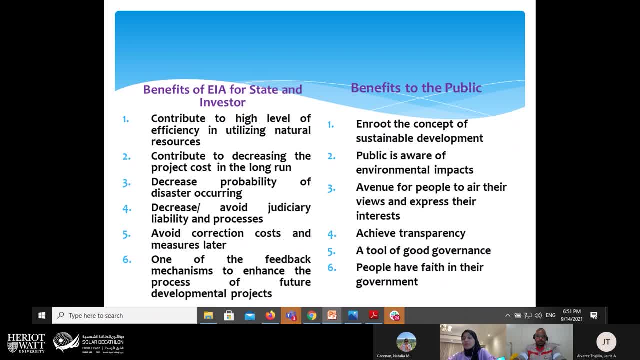 decrease the cost from the first run And also it is decrease the probability of disaster occurring and avoid also judiciary liability and processes. Also avoid correction costs because it is deal with by it is work as proactive approach And about the benefits to the public. it is. 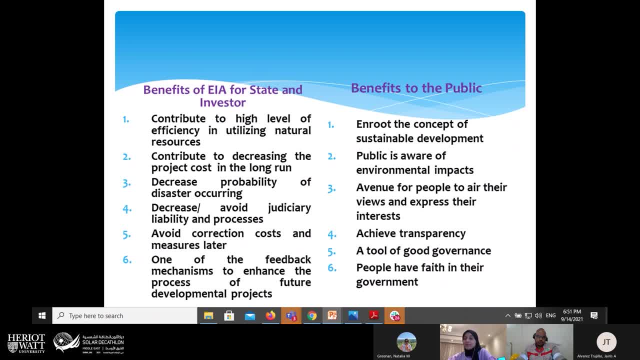 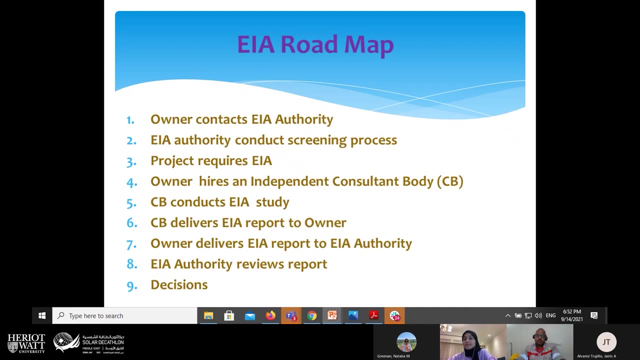 a lot of benefits for actually for the public. It could include the concept of sustainable development and also make sure the good consultation and good relation between the government and also the owner of projects and the public itself, public themselves. So when we talk about environmental impact assessment, we need to know how we could apply the EIA. 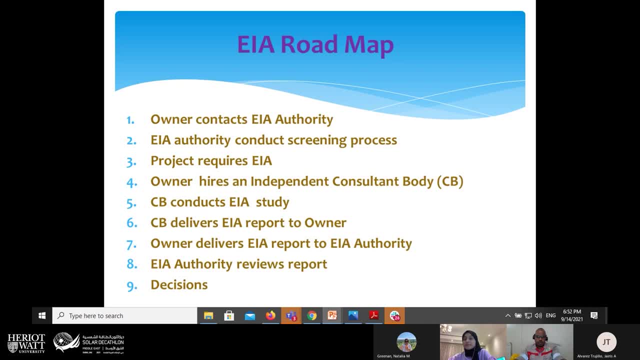 So this roadmap talk about the implementation of EIA. It is a symbol. The owner contact environmental impact authority. The authority conduct screening process. This is the first process in the EIA. Then, if decided to that the project need EIA, then we will go to the other step of hiring consultant body. 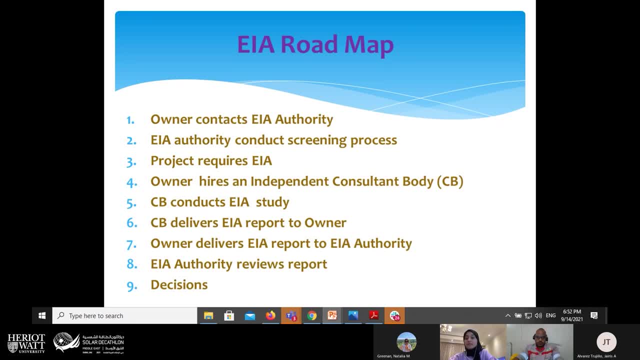 to conduct the EIA After hiring the CP or the consultant body started immediately. the consultant body started immediately on conducting EIA, then deliver EIA report to the owner. The owner by himself take the report and send it to the EIA authority for reviewing and taking decisions, As we talked. 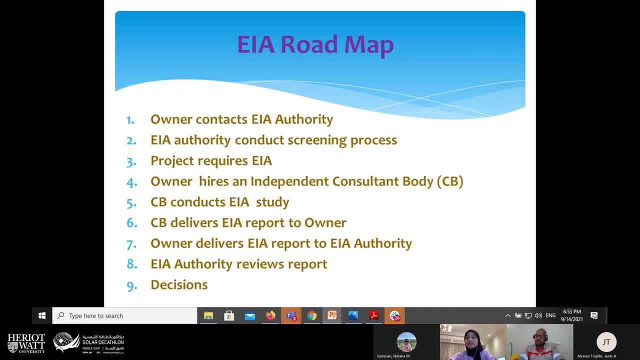 before. the decision could be either to take this project or could not take it. Sometimes the EIA decision or the EIA authority decision came with to take the decision. but we need- we have- some mitigation plan to reduce the impact for the EIA. 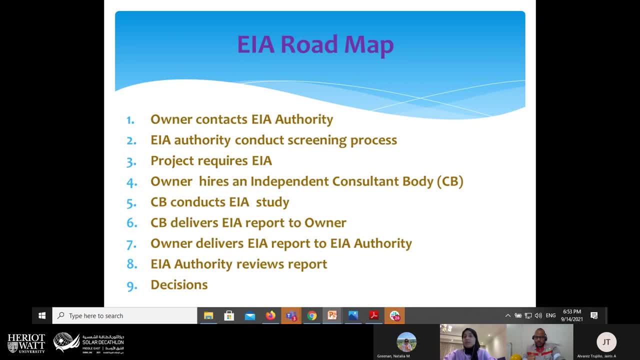 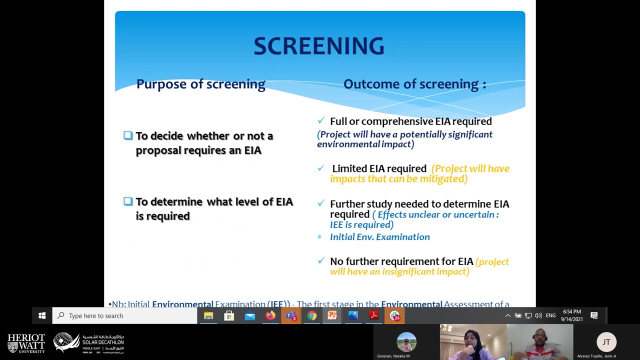 the environment. so it is a proactive way. when we talk about projects implementation and project applying, we need to know that or predict the impact before the start of project, then have suitable mitigation plans. so when we started with the, when the eia authority started the process of eia, first step will be the screening. the screening is like to refining the or. 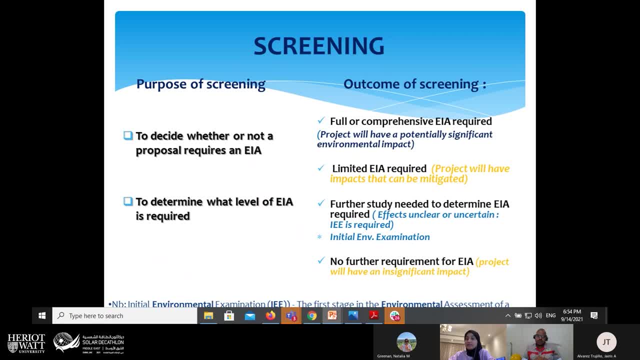 take the desire decision about the proposal itself and also determine what level of eia is required. as we talked before, we need to take to, to take the decision either to if there is severe or extreme impact. so maybe the authority decide that to not take the project, but sometimes when 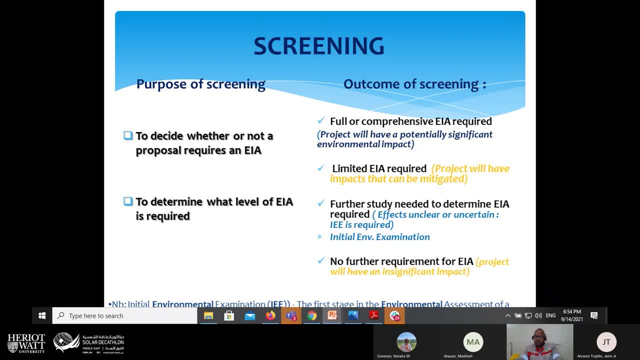 when they find the impact not very severe, major or minor, they can take the project with a mitigation plan, as we said. so the outcome of screening: full of comprehensive eia required. number one, this one. this is one of the outcome of screening. maybe also the outcome will be: we need limited eia required. 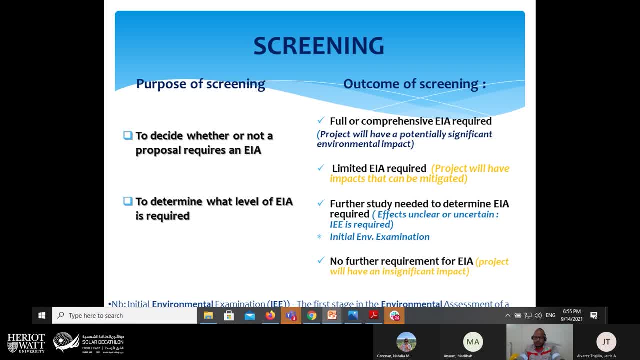 or we need further study as environmental examination, initial environmental examination, to decide either we need to take the, either we need to conduct the environmental impact assessment or not. also, one of the outcoming of screening is ��서, the eia. can we, can we can experiment a little bit. what is correct? 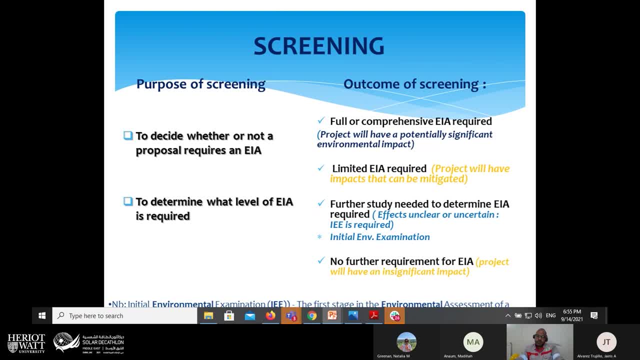 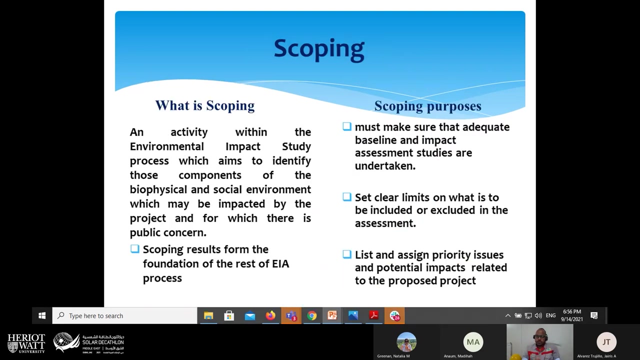 to say- and that's what will be very important for the survey: so when we have the eia for so it's doubts, either the project need EIA or not. After we conduct the screening, now we have the decision- we need to conduct environmental impact assessment. The second step will 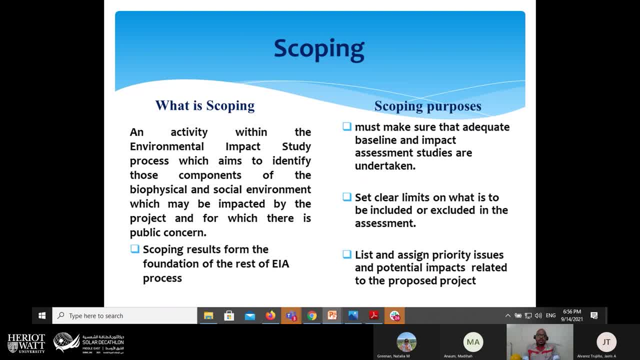 be the scoping? The scoping is activity within the EIA study process which aims to identify those components of the biophysical and social environment which may be impacted. So it is by this way we could reduce the cost, reduce the time We know. 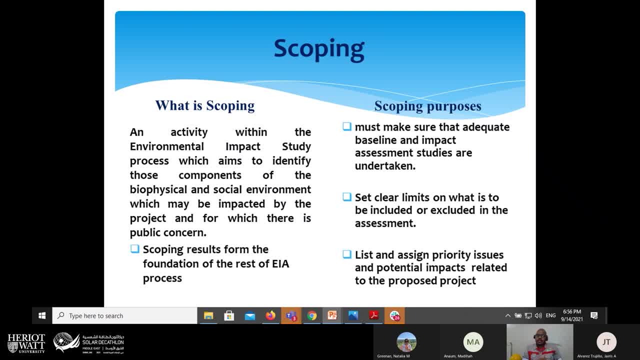 about what impact exactly we're going to study. We know exactly what impact, what the severe impact we need to focus on during the impact, during the study and also we during the scoping. usually we we explain the information we need to, the information about the project, as at the beginning and then also 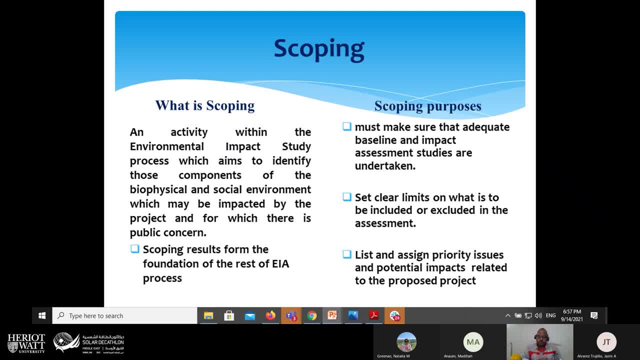 explain the baseline of the environment. What about the baseline? The baseline is the, the environmental condition for at the beginning of the project. So it is very essential: The baseline of environment of the, the project area. It is very important because we need to then. 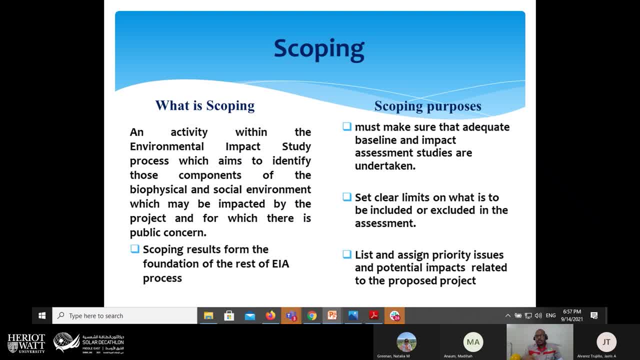 at the end we need to evaluate the impact of the project activity. So the scoping is one of the important steps. on the in the EIA It is set clear limits on what is to be included or excluded, and also it's list and assign priorities. 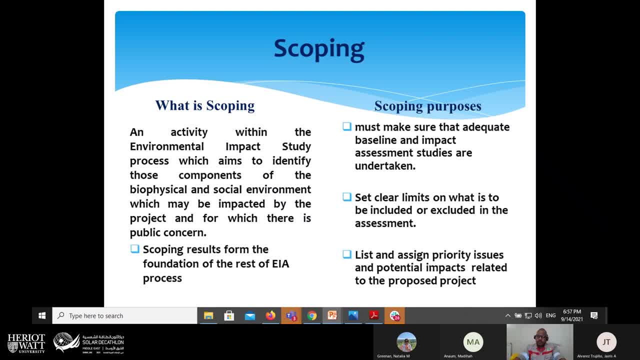 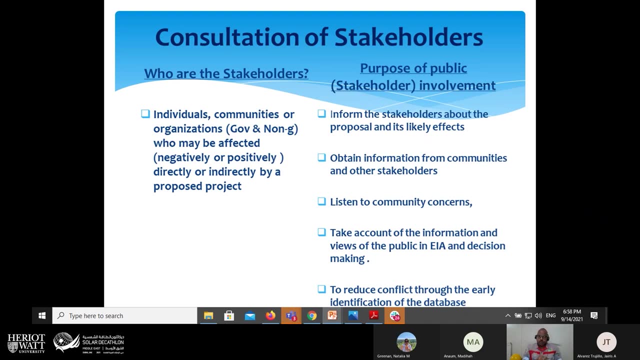 for potential impact and for the evaluation needed for each impact. The the evaluation needed for each impact. After conducting scoping, we move to consultation of stakeholders, These very important steps we need to to this. We know stakeholders usually consist of individuals, communities. 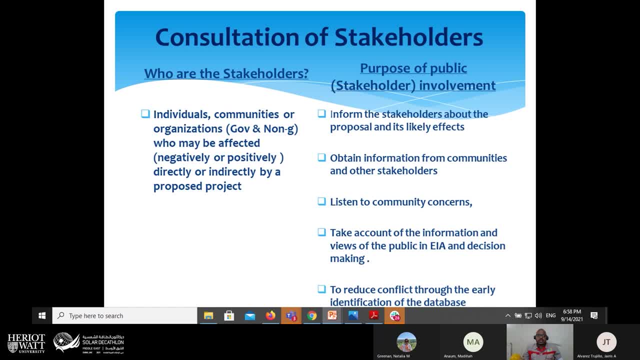 organization, government or a non-government organization- Any party will affect negatively or positively by the project. There are stakeholders, So the stakeholder consultation is very important because we need to make a good relationship between the owner and the government and also the people and the public. Also, we need to take information from them and also give. 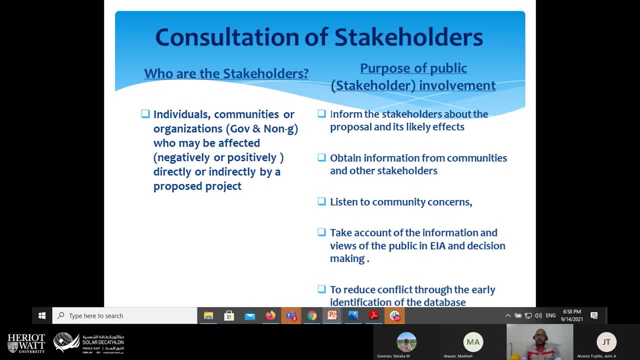 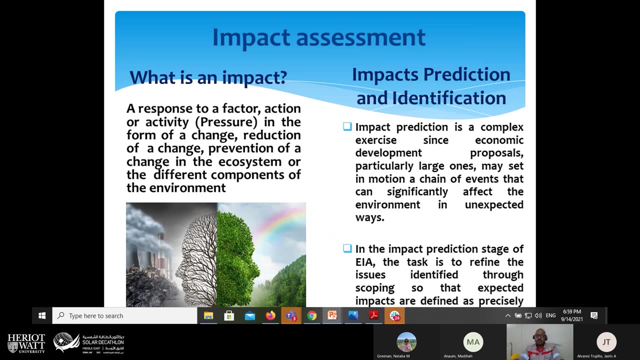 them information about the project impact, because they will be impacted by these activities. So we need to consult them. So we need to consult them at the first of the project, at the first steps. Then we move to the essential and significant step of the EIA, which is impact assessment. 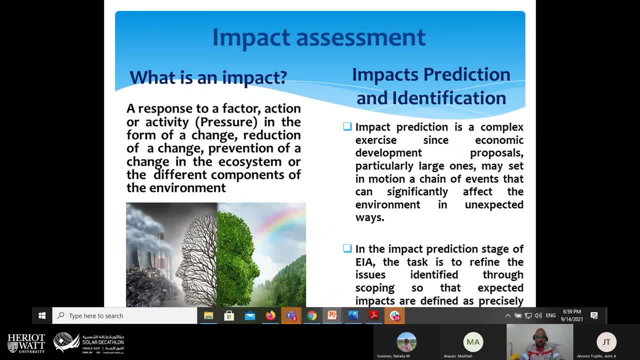 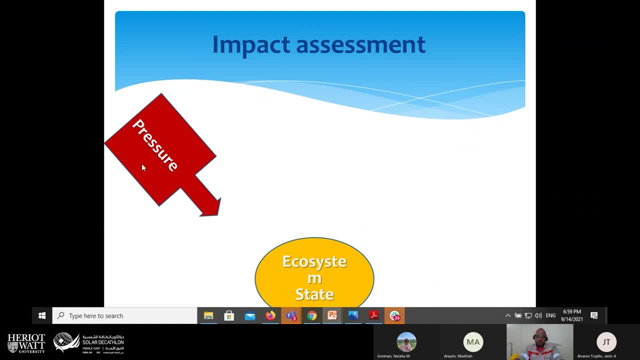 The impact is a response to a factor, action or activity, pressure like this: This is the ecosystem and this is the pressure. the activity of a human being, The project itself, Construction operation and so on. Then we have the impact. 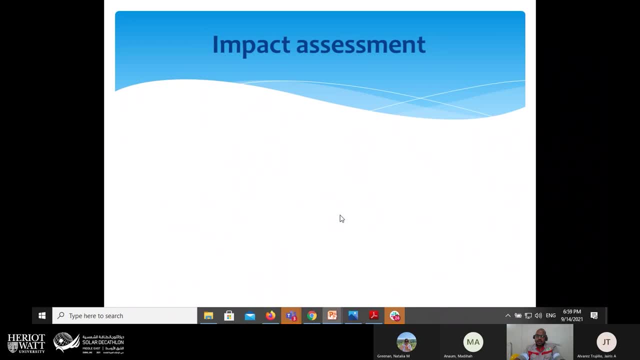 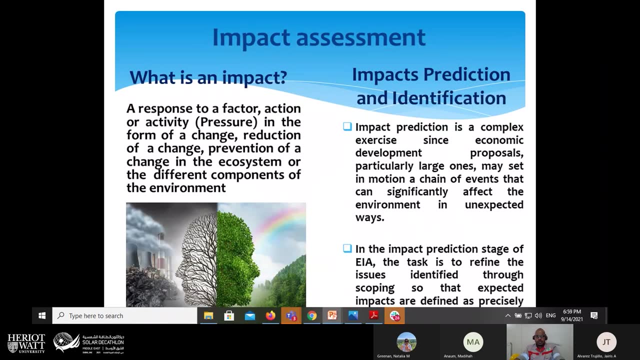 So it is as we can define it. It is sometimes a change or reduction of a change or prevention of a change in the ecosystem. Ecosystem is a very balanced system. from the gut It's game like this, So any change in this ecosystem could have adverse impact or positive impact. 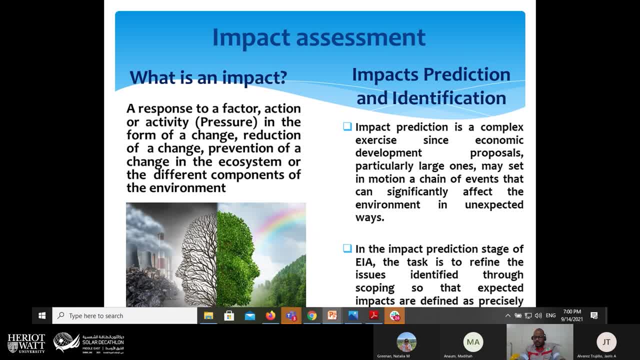 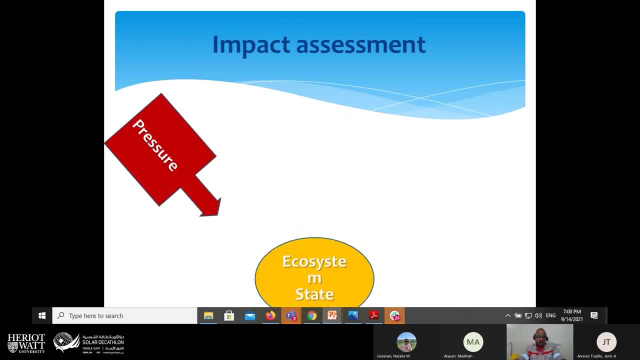 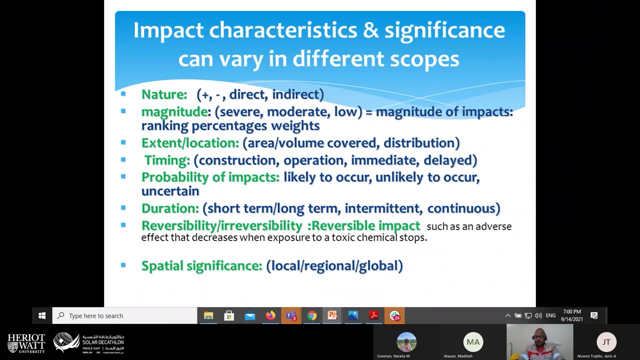 Our roles here in impact assessment: to predict the impact and identify the impact, to identify then the suitable mitigation measures for those impact. So the impact characteristics and significance can vary in different scope. The nature of impact is very from direct impact or indirect. magnitude of the impact: severe, moderate. 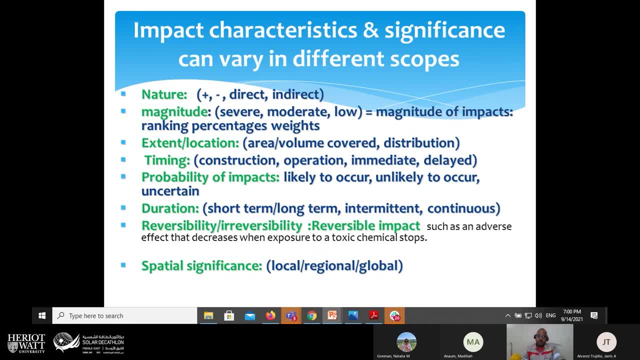 like this: extent, location, because there is some impact, have specific volume and distribution is vary from impact to another. So we need to know the extent, location, the timing during the construction phase, operation phase, during the project phases, Generally we need to know about it. 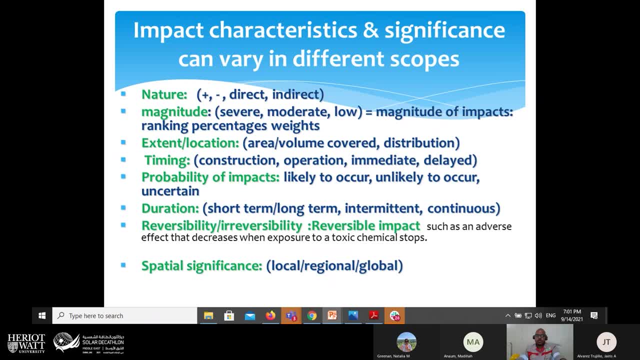 Probability of impact likely to cure. unlikely, like this duration. It is about long term, short term, continuous impact and so on. Reversibility and irreversibility, because we could take example of reversible impact, such as an adverse effect that decrease when exposure to a toxic chemical stops. 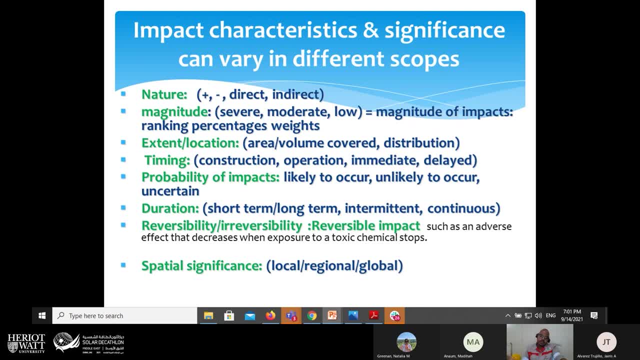 When this stops, then the impact reverse to the normal state. So it is- we could call it reversible impact- Special significance, like the local, regional and global. We can take the acid rain as an example, because acid rain usually had a regional impact. 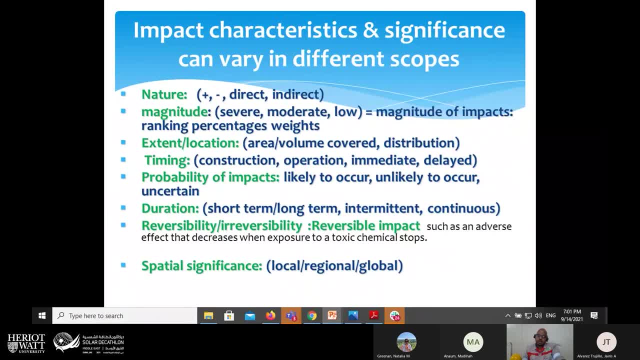 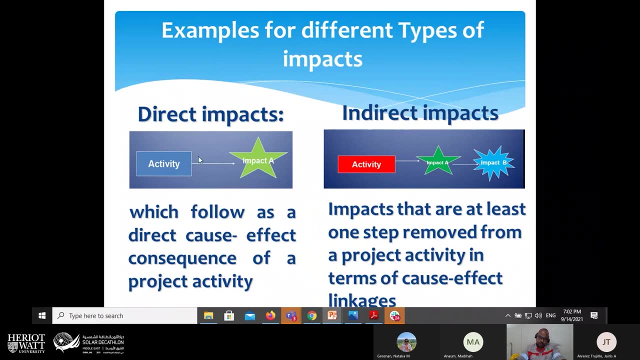 It's good, The emission could happen in area and the impact could happen in another region. So we need to know about spatial significance, about example of direct and indirect impact. We could. it is, it is very direct, It's very clear: activity cause some impact. 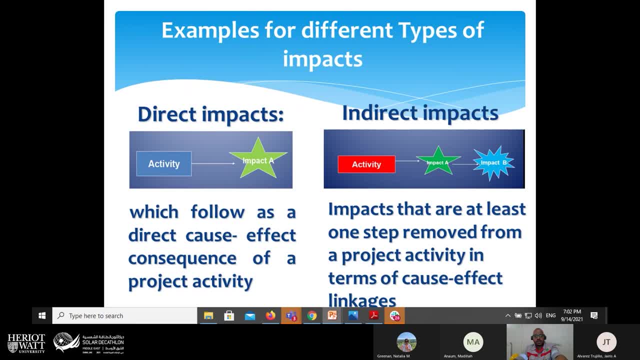 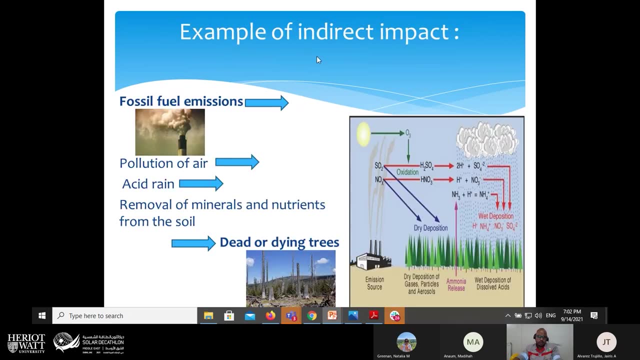 Emission, like emission of toxic gases, have impact in the bird And the nest of bird and so on. It is a direct impact, Indirect impact that's like acid rain. We could take some example here for indirect impact: fossil fuel, The emission of fossil fuel. 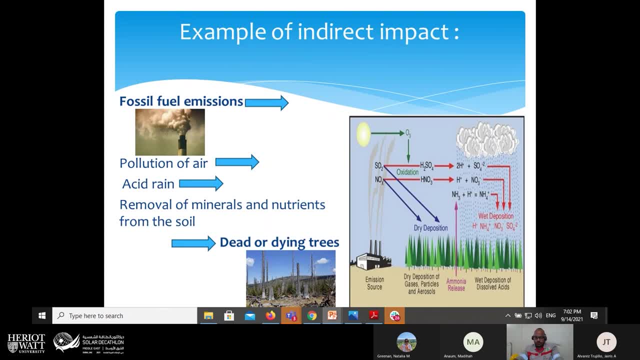 Could have impact of pollution of air. Then acid rain could be formulated by form, by The chemical Reaction. we could have H2SO4 or HNO3. So this acidic Component could react and could react with the air and could precipitate in the 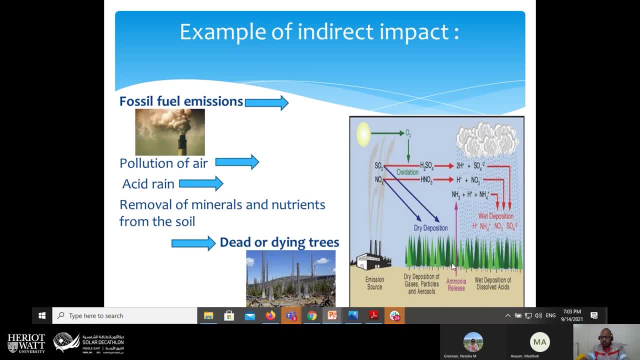 Environment, causing wet deposition for the, For the, For the Trees and like this. So this could, If Eventually, lead to dead of trees and vegetation. So the dying of trees and affecting the vegetation Could be indirect impact of the emission of fossil fuel. 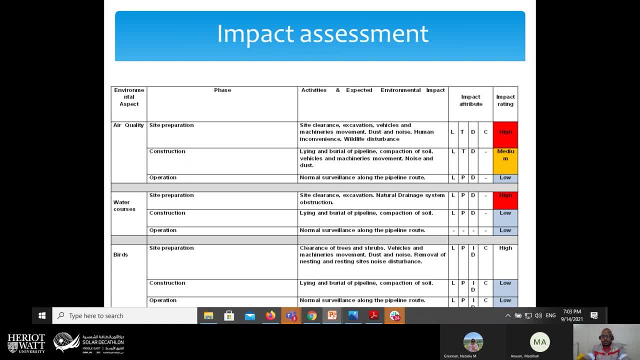 Then we need to know also about the impact assessment, because we need to add the report of the EIA. We need to identify Some, Some Impact and also identify all the impact and assess those impact, like this schedule. We have site, We have environmental aspect, like air quality, as example. 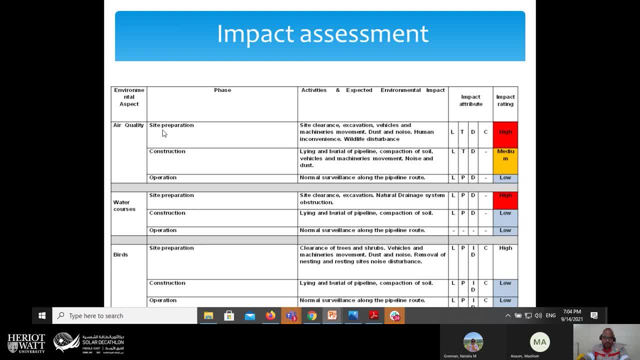 We take the some one phase as site preparation as example. Then we evaluate the impact on the site. Preparation of project could be site clearance, excavation vehicles. This is activity of excavation could lead to some movement or machineries. movement or the activity of machinery. 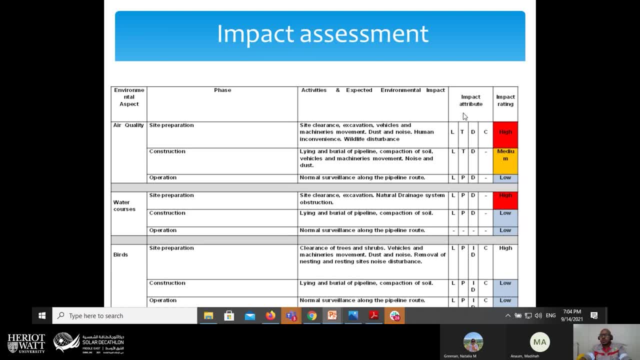 Movement could lead to dust and noise. This is the impact. So we need to know about the impact attribute, like the, If it is local or regional, like this. L mean local here. If it is, We need to know about also If it is. 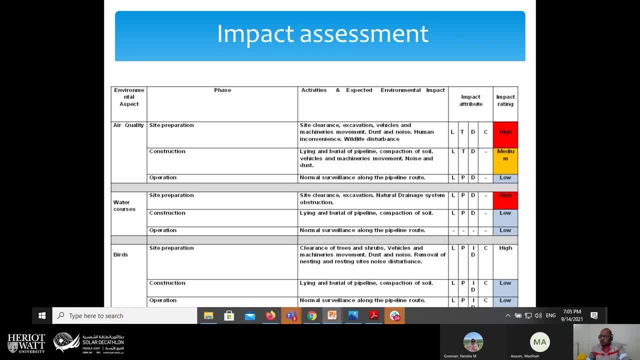 Direct impact or indirect impact. We need to know the different about the different attributes of the impact. So usually, as we can see here, There is some, Some, some attribute. We need to assess the impact depending on this attribute. See usually refer to cumulative impact. 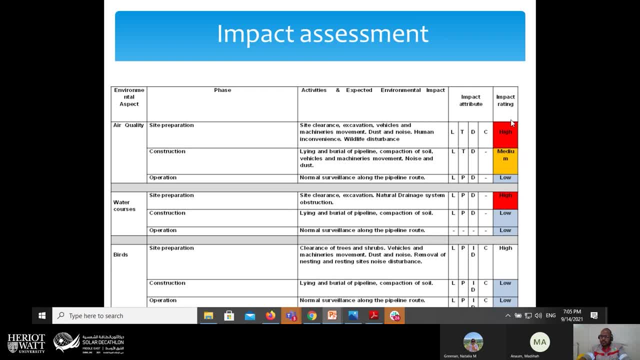 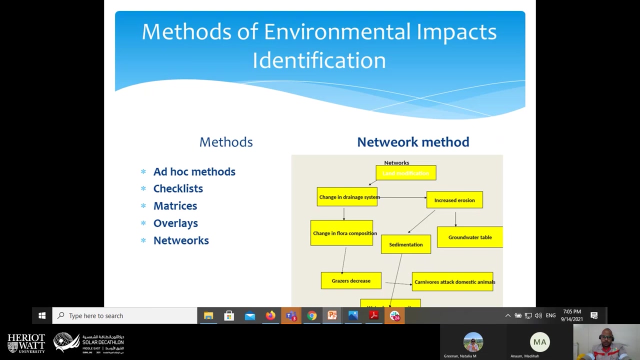 And also here, impact rating, talking about the severity of the impact. This is high, medium or low. Depending on this rating, we could decide about the mitigation, the suitable mitigation measures At the end. we need also to know there is some methods of environment impact identification. 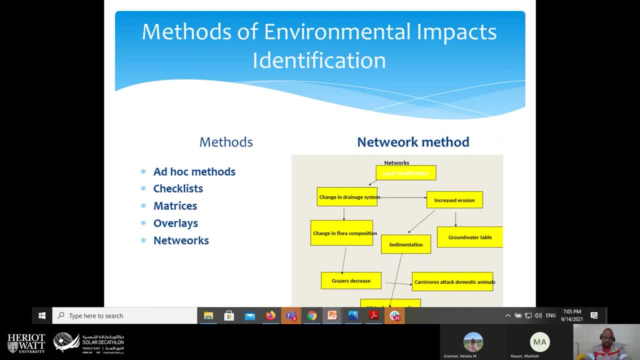 Method like ad hoc checklist, matrix, overlays and networks, Usually ad hoc checklist similar. It is used for deciding about a list of impact and it is good for site selection and so on. And also we had matrix Matrix have a lot of advantage, like it is a link action to impact. 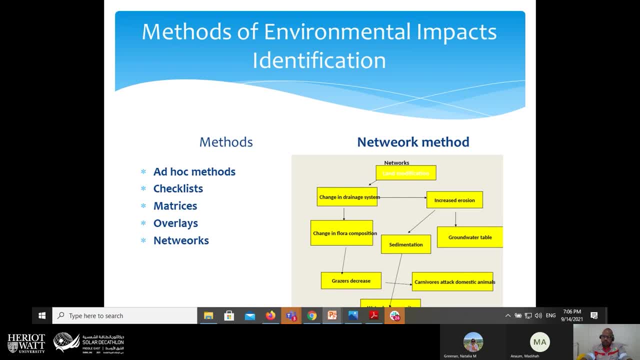 And also We had matrix Matrix have a lot of advantage, like it is a link action to impact. and also We had matrix Matrix have a lot of advantage, like it is a link action to impact and also Discipline the EIA result perfectly. 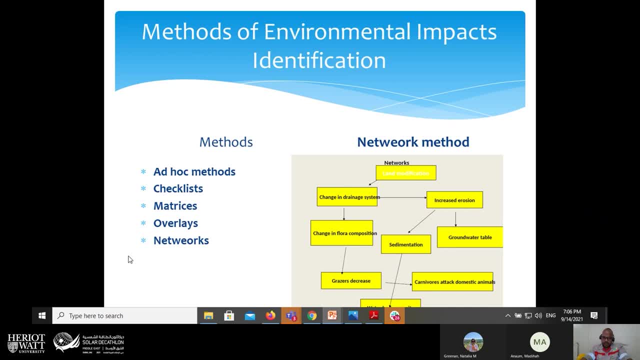 So it is. I really enjoy to use matrix method in evaluating the impact For the project contain a very major impact and so on, And because it is also have, it is very clear on description of the impact and could give you Good overview for the impact. 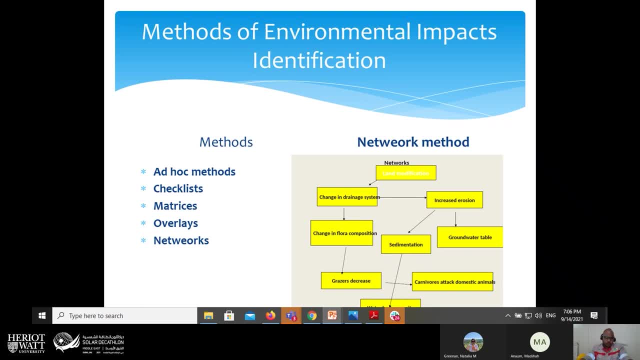 But we can also check. there is other method, like overlays. It is used a map for, For discussion, for describing the impact, and now there is Some improving in this method, like GIS methods and so on. So if we take the network method as example, one of the examples we could, 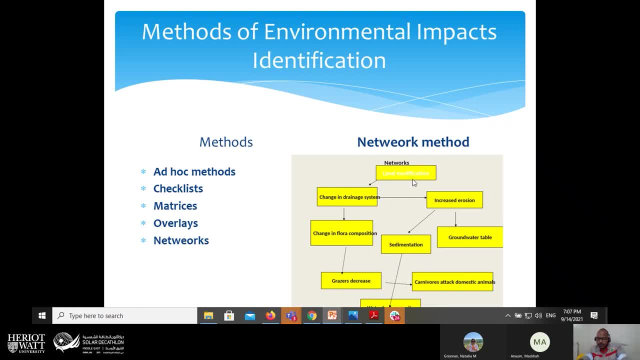 See here the land modification Could this activity could lead to change in drainage system as example. This direct impact then change in Florida composition. This is indirect impact of land modification That this could lead to grazers decreases and eventually to attack of domestic animals. 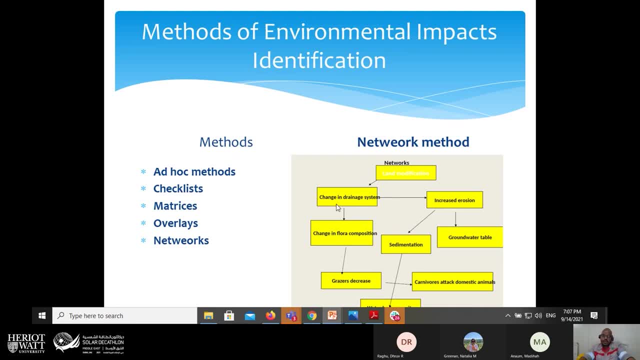 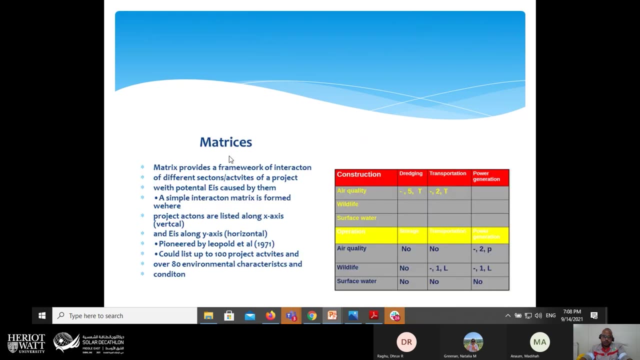 This is one of the example of how We could link the impacts together and the. so this method is very useful To describe that direct and indirect impact as general. We could take also the matrix one here we could talk about The face, the project face, like example construction. 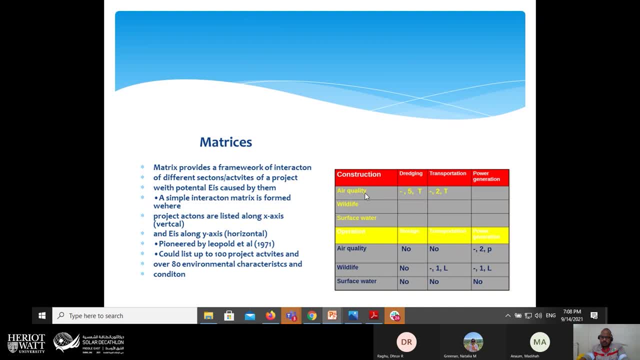 Different. there is a different criteria like air quality, Wildlife, surface water- we could take example of air quality during Drinking. we could have some negative adverse Impact of air quality, some toxic release of Of the machinery use and also the impact. we need to assess the impact. 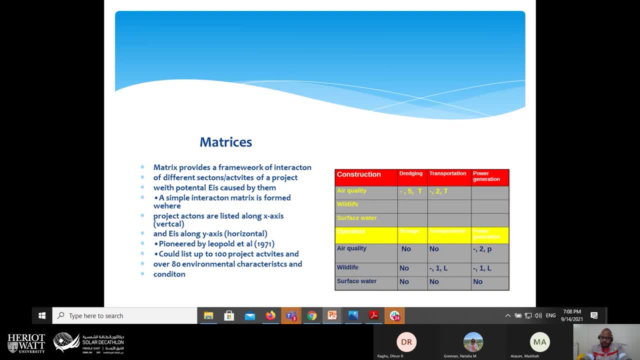 From 0 to 5 as example, and also We need to identify also the Continuously of the impact. so Usually we use this, This method for For for evaluating the general Evaluating the impact in a lot of projects, like 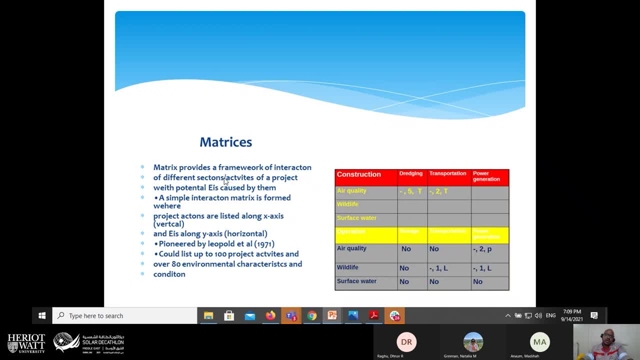 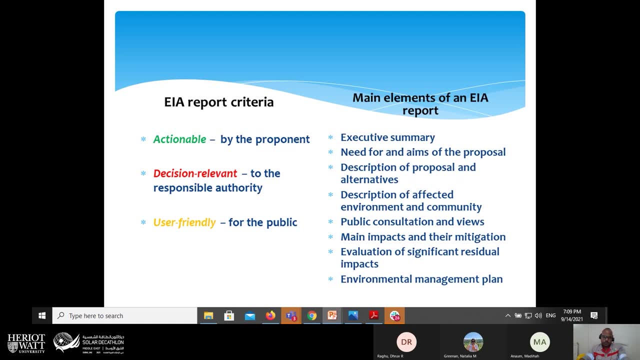 Oil and gas and so on. it is depends on the assessor itself. He could take the best method he could use for assessing the impact. At the end, we need to make the EIA report. The report should be actionable, decision relevant and also user friendly. 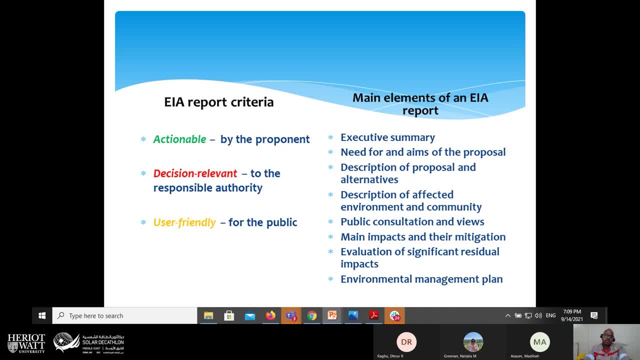 We need to collect all those data to make our final report, Then send it to the EIA Authority to decide about the project. So all this, as we talked before, it is Applied by the consultant body. All these steps is after the screening. 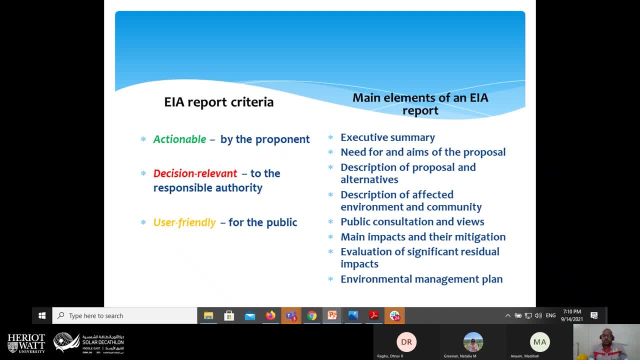 Like scoping consultation of Public and also The impact assessment itself and then preparing the report. It is the responsibility of the EIA consultant body. The consultant body at the end make the report By ensuring some executive summary Need for an aims of the proposal. 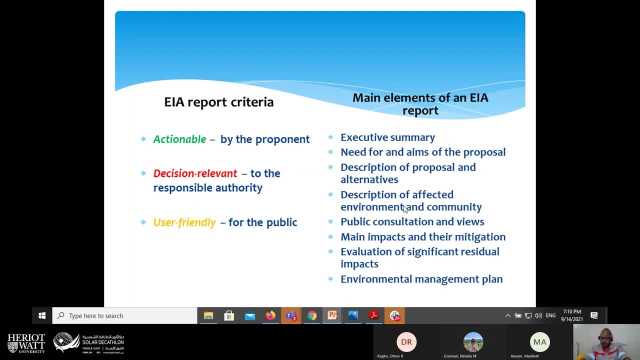 Description of proposal: description of affected Environmental and community Public consultation results, Main impact and also evaluation significant Of significant residual impacts. and at the end We need also to the consultant body, Need to make some environmental management plan. This plan have included, should included, the mitigation measures and so on. 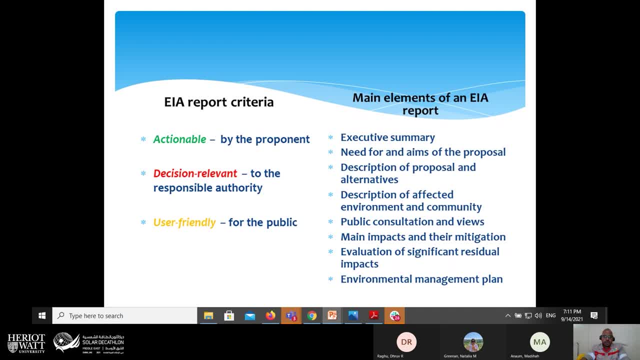 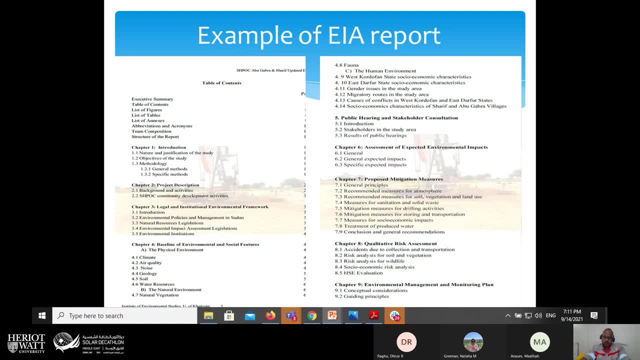 This is an example of real life And also the report conducted, depending on conducting, conducted The EIA conducted for the oil and gas project, For our site it is about. it is just here. We shared the content: summary introduction, project description. What about the project itself? 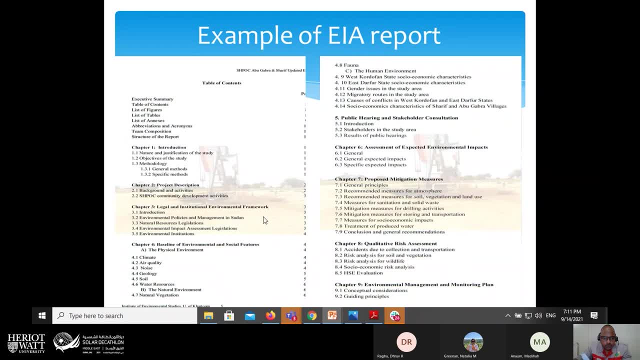 The legal and Legal environmental framework and also the baseline should be Made Measured here, should be measured and should be Mentioned here because, as we talked before, we need to Evaluate the impact after this baseline, After the activities of project going on. 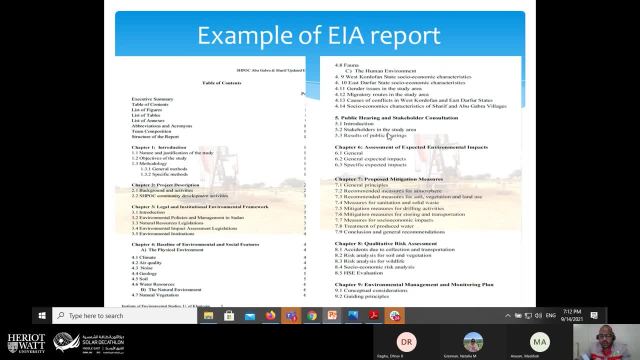 So we need to refer to this baseline And then the consultation. here We find also the assessment of expected environmental impacts And then Suppose mitigation measures and sometimes added qualitative risk assessment. At the end we will find the environmental management and mitigation plan. 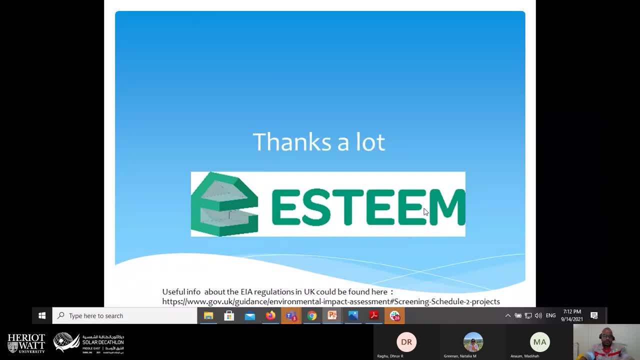 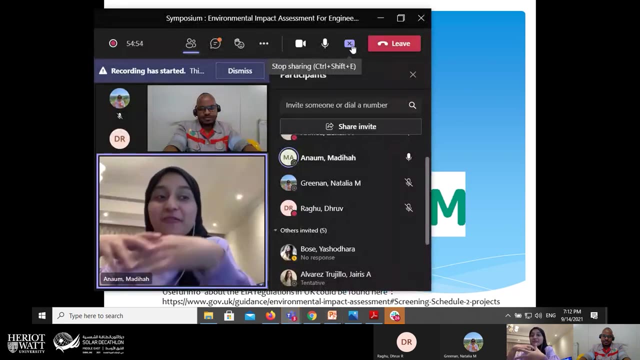 Thank you for attending and that's all from my side. If any question, I'm happy to answer. Thanks a lot. Yeah, Madiha, That was indeed a very descriptive and informative presentation. Um, Um, To optimize the project potential in order to yield good results. 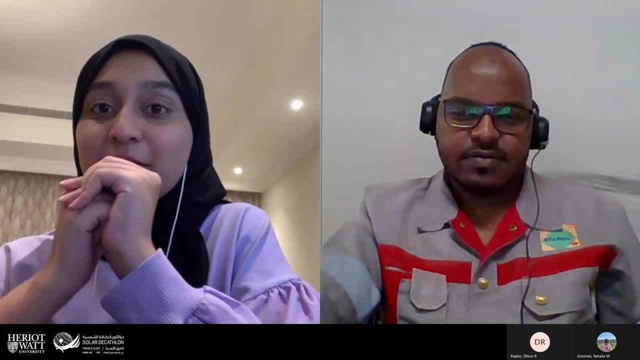 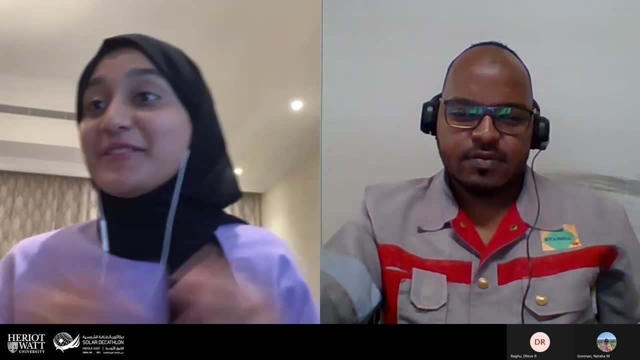 Like really important to conduct an EIA to you know, To ensure the project is sustainable. Um, So thank you so much for sharing some light on that through this useful presentation today. All right, So moving on the question answers session. now We have received a couple of questions in the registration forms. 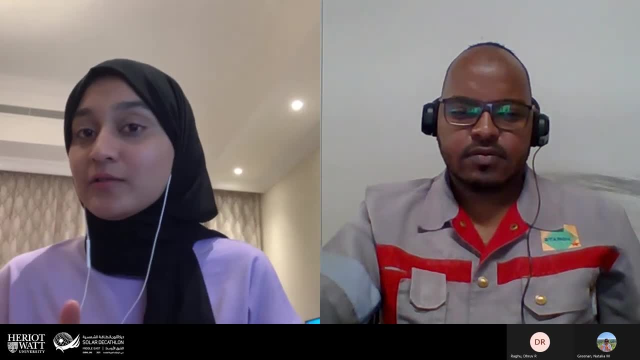 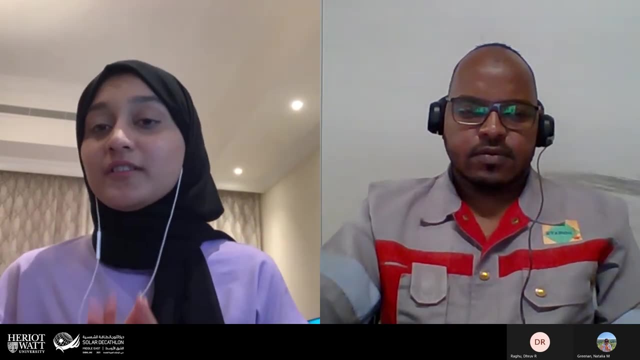 Which I'd like to ask you, Zuhair. at the same time, Anyone from the attendees can also ask questions by raising your hand Or typing it in the chat box. So, Um, The first question is: what are the factors affecting EIA? 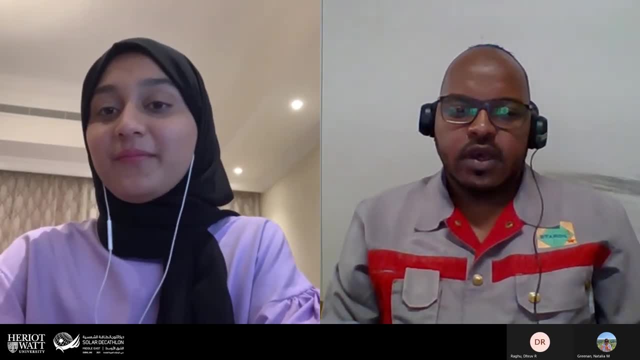 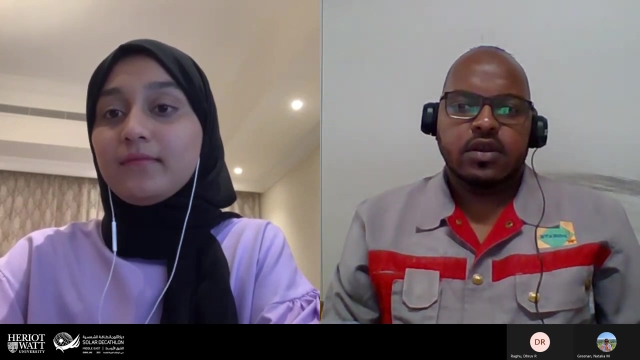 Actually, it's very important question and also very big question Because a lot of factors could affect EIA, Like the consultant body itself. If the consultant body is competent could affect the EIA positively And if the EIA consultant body not very competent, the EIA report could be affected. 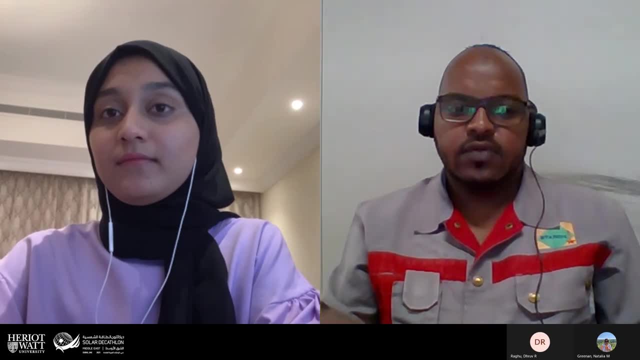 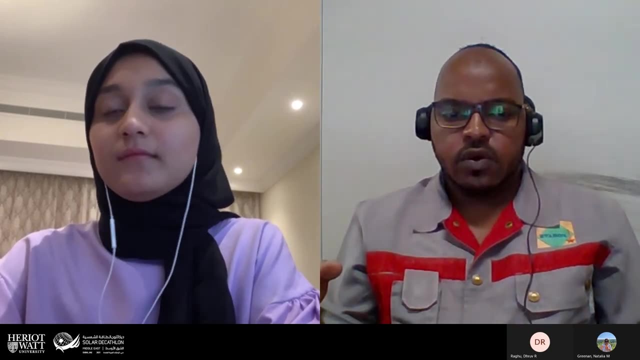 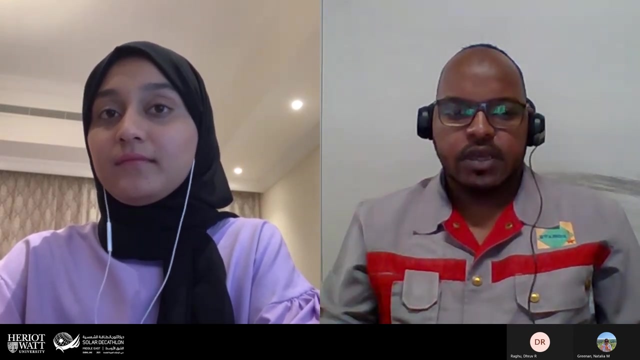 Also we could Move to the next step, The screening. If the screening not applied very by competent way, So could lead to elimination or stopping some essential project. It is a very significant decision, So the authority itself decision could affect or the competence of the authority itself. 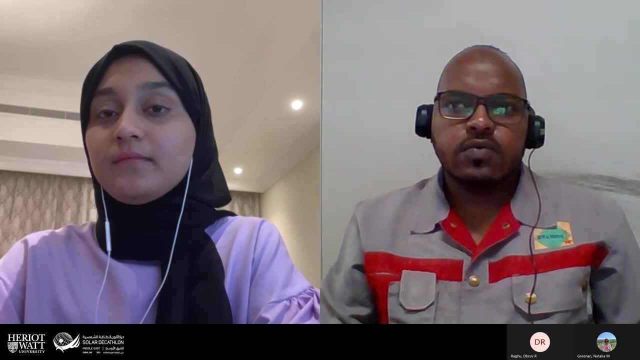 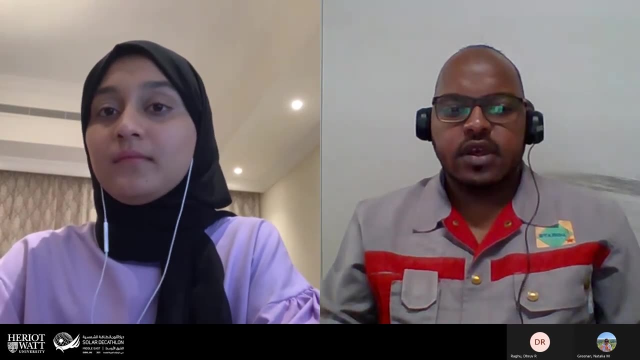 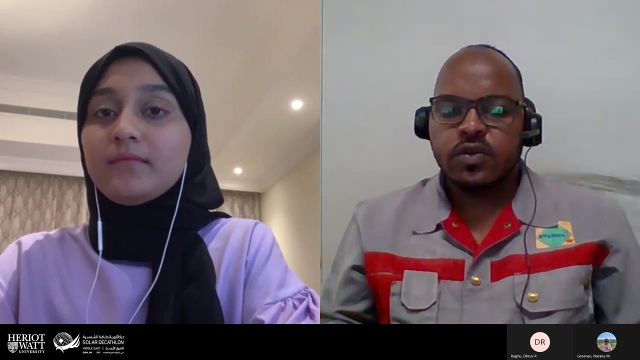 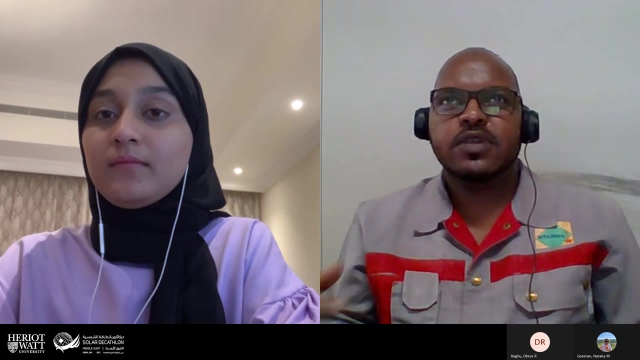 Could affect the EIA And also very essential effect could be from the consultation, Because if the consultation steps conducted perfectly, So we know about the social economic effect of the project itself. But if it is not like very deep, Sometimes they do. 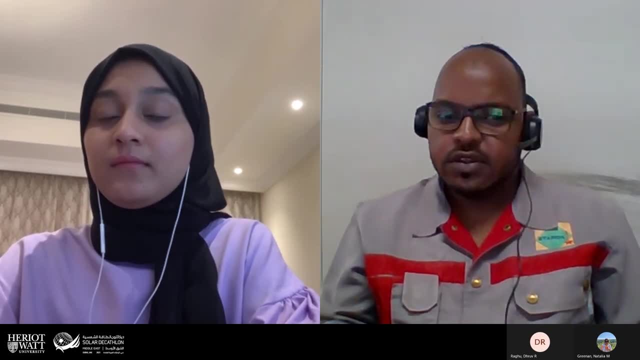 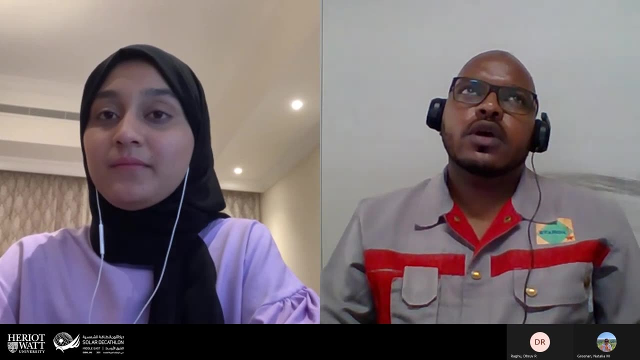 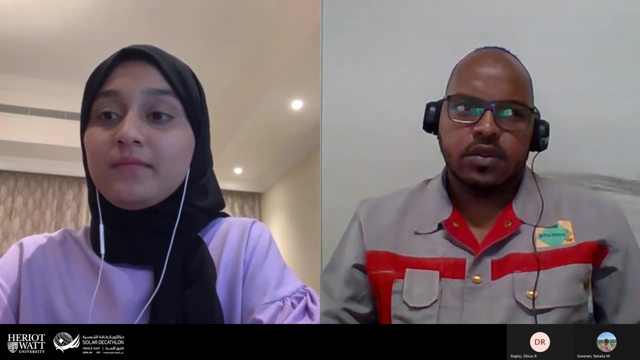 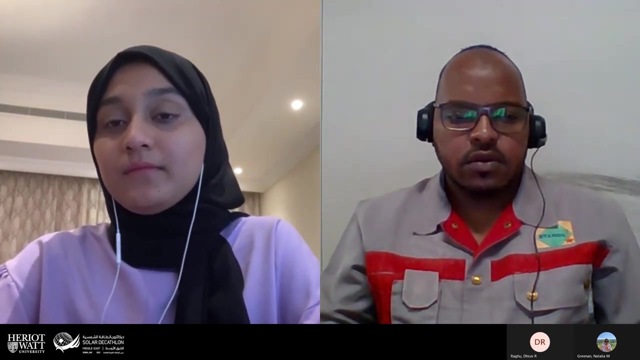 They did it very quickly And not focusing on the consultation of people And not hearing from them, So it's good effect. Another also factor could be the time, Because sometimes the time very limited, So they conduct the EIA very quickly. 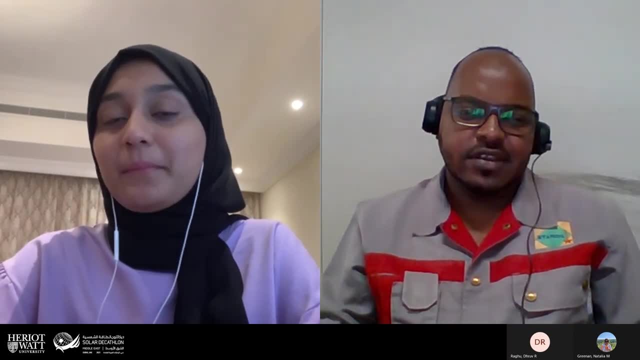 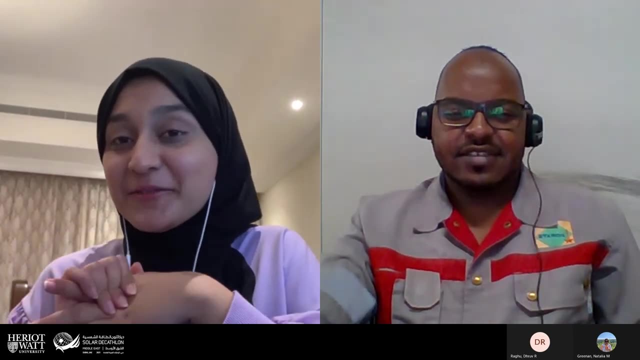 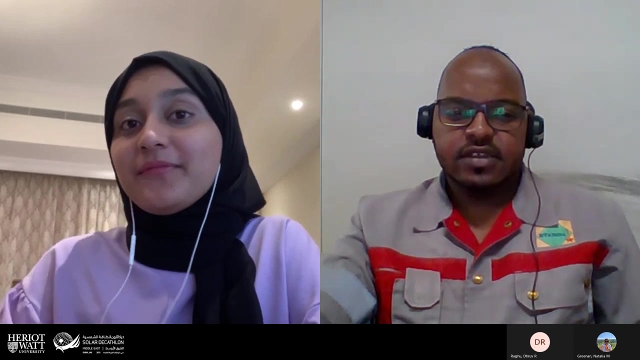 So the result will be not very accurate. That's, briefly, All right. That was perfectly answered. So our second question is: What do you believe is essential for in an EIA? in your opinion, The essential steps. What is the best method for, like environmental impact assessment? 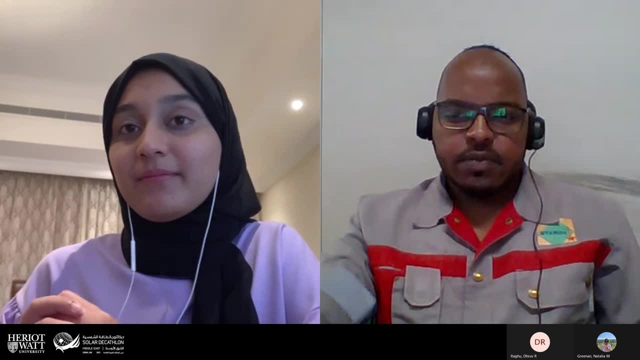 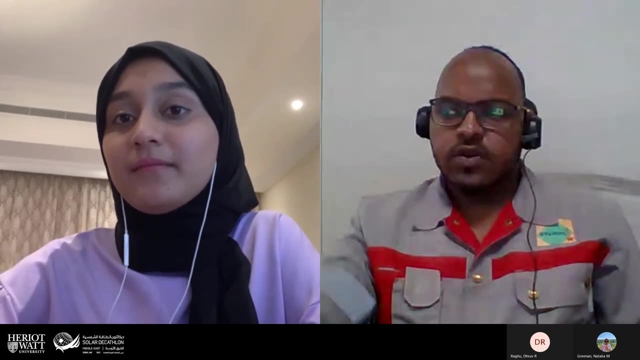 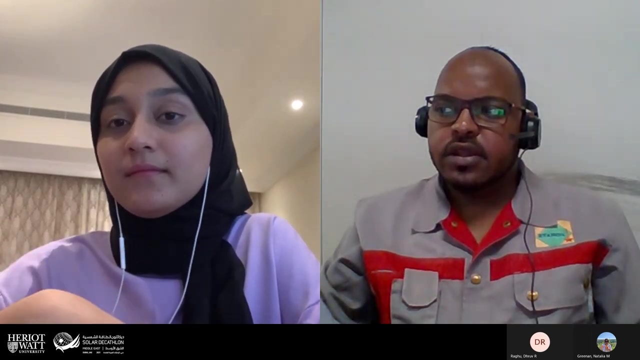 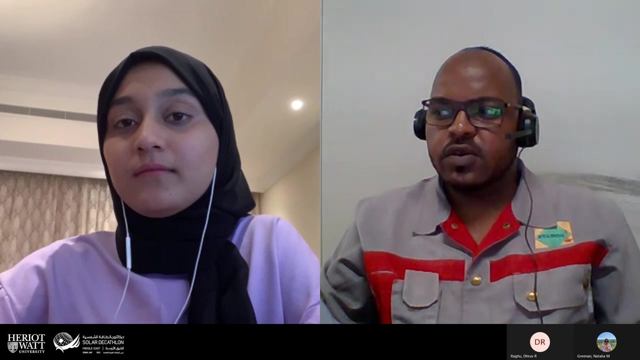 Yeah, Yeah. For evaluating the impact, I do use usually the matrix method Because it is usually linked- the impact with the activity Itself, And also the matrix give you some space to talk about the relation of impact together And so on. 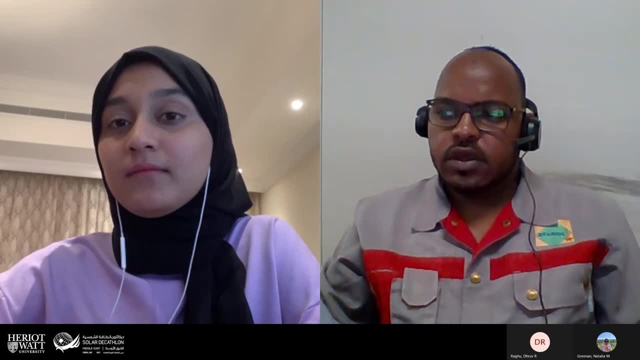 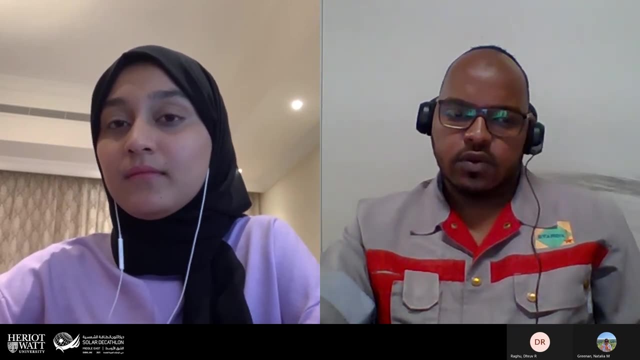 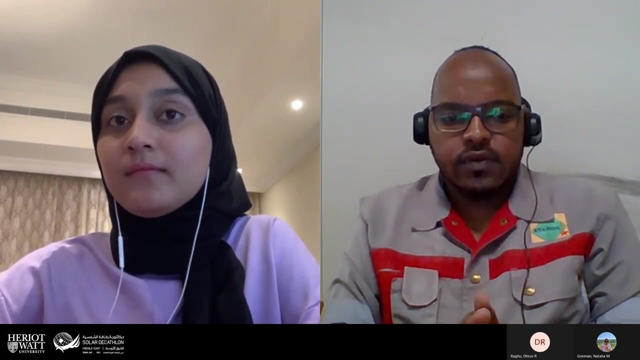 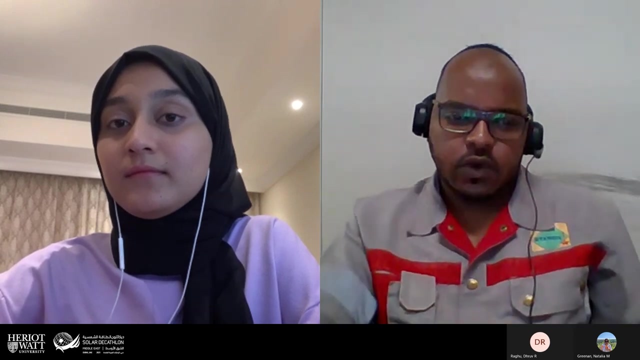 So I do recommend to use matrix one Also because it is good for displaying the results. So it is very recommended by me. But it is depends on the in the impact. So it is very important to evaluate the body or the consultant body to take the best method for evaluating the impact here. 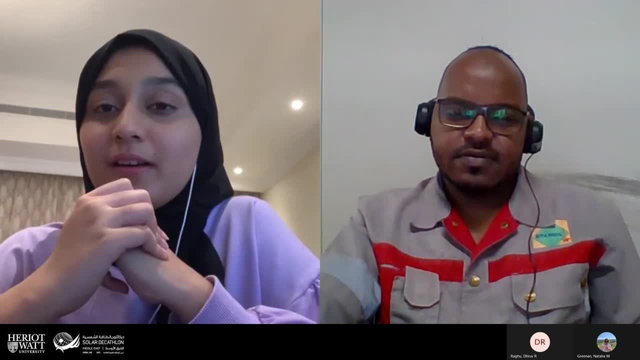 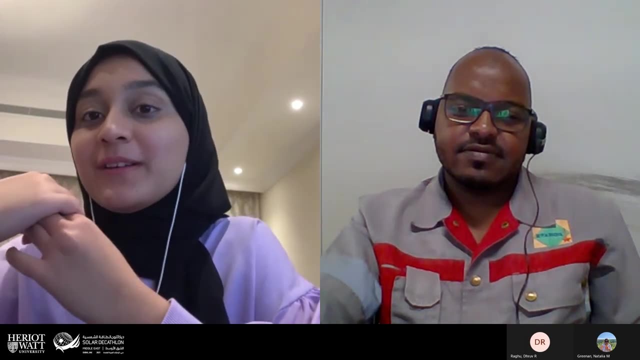 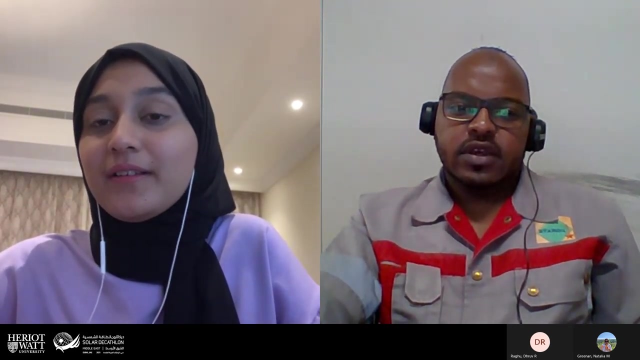 All right. So has environmental impact assessment contributed like enough to the protection of our environment? Like, could you like give us like a live example for that? Yeah, Actually, at the oil and gas field. I can take it as an example. I can take it as an example. 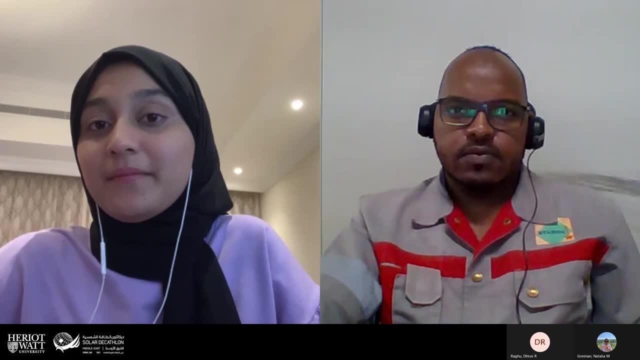 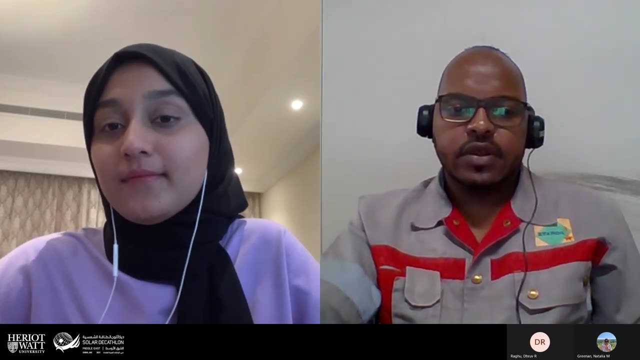 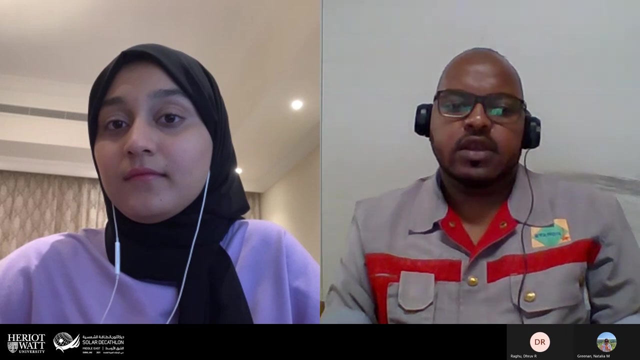 As there is some mitigation plan, lead to know about what exactly we could focus on during the project. Because they do, you think, that they take all information about the baseline, or fauna, flora, anything about the area itself. So when you compare it to the activity or the 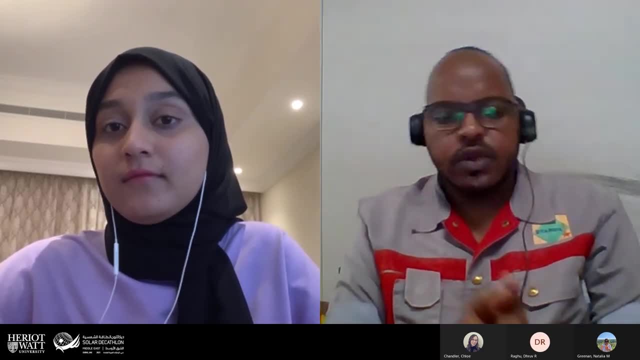 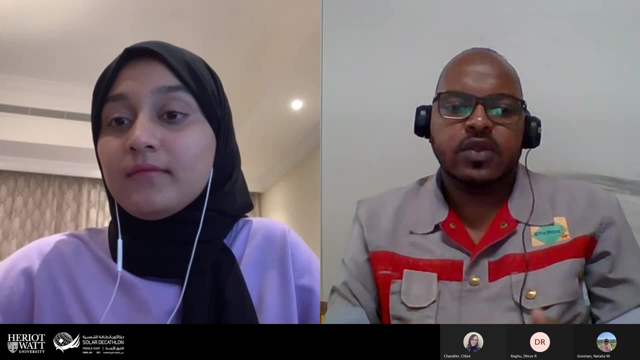 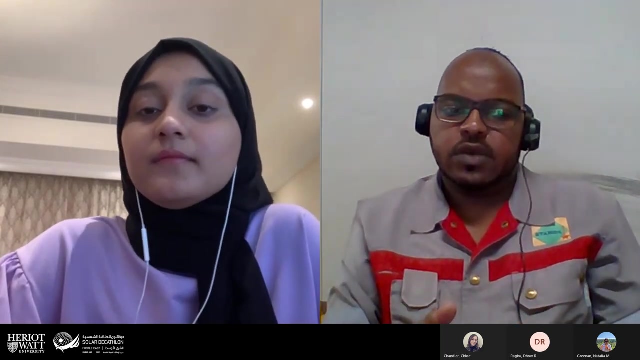 uh, the the environment after or during the project. you could- uh, usually we, you will take quick action and also proactively- uh, proactively- you can take the suitable action to avoid and to mitigate the impact. so it is very helpful actually, and also there is some international cases of 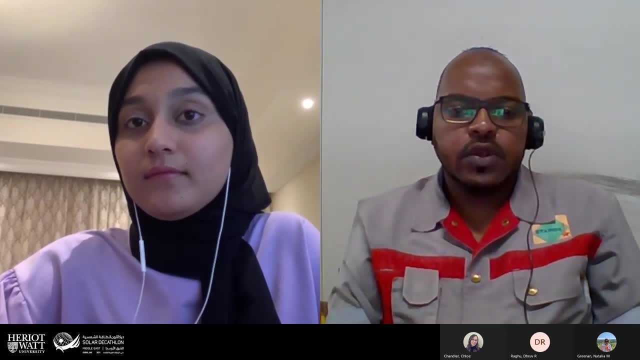 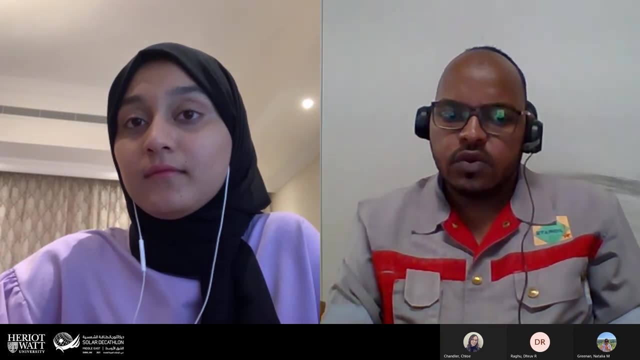 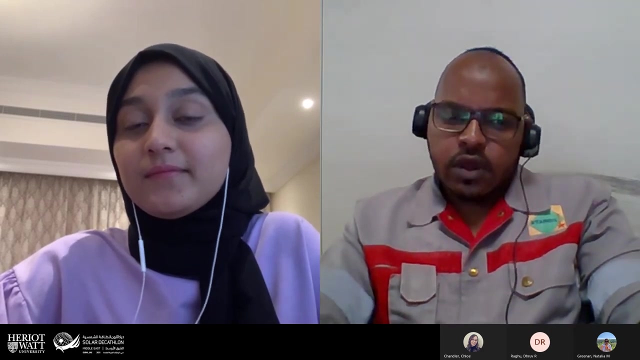 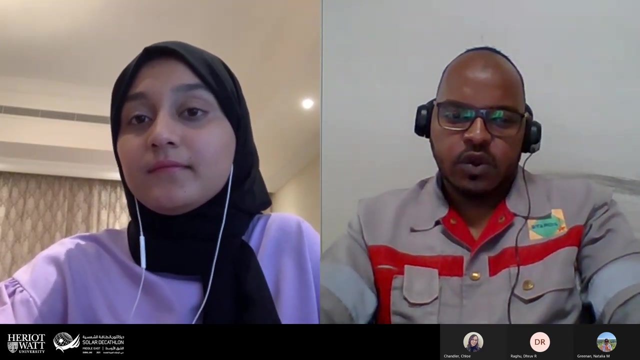 stopping some project could lead to a very adverse impact to the rivers itself and and so on. so and also for the weather, for the acid drain causing and so on. so it is very effective way we could use it to reduce impact and also reduce the cost, as we said before. 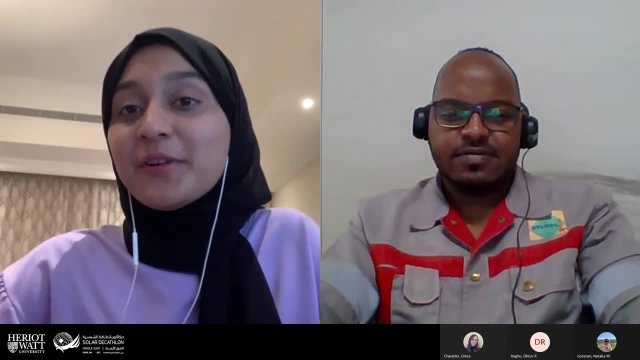 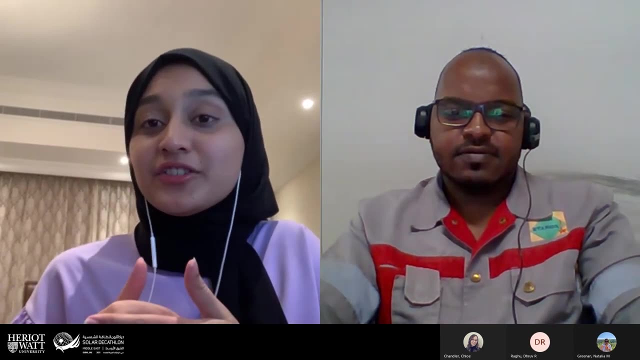 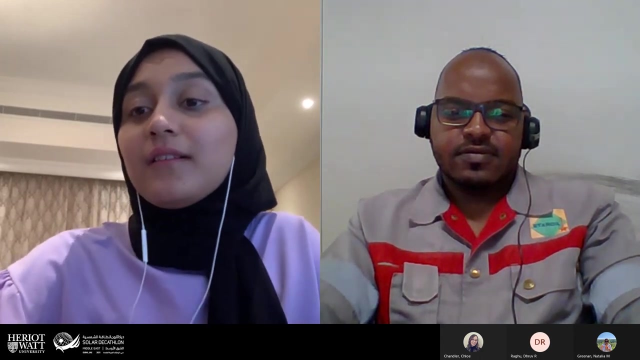 yeah, thank you for answering that question, um. also coming to our last question for the session: any advice that you would like to give to someone conducting an eia and what are the challenges, did you like? what are the challenges you faced while conducting an eia as a health officer on field? actually, the, the, the real challenge when you're consulting the. 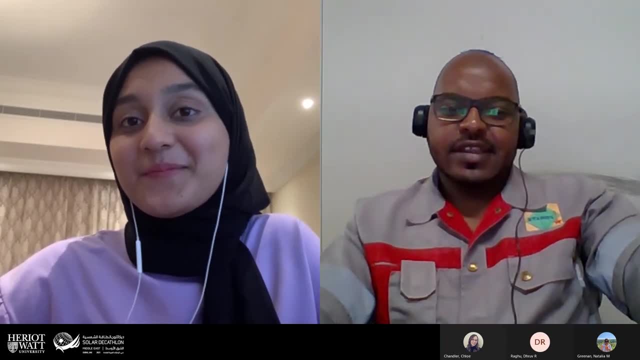 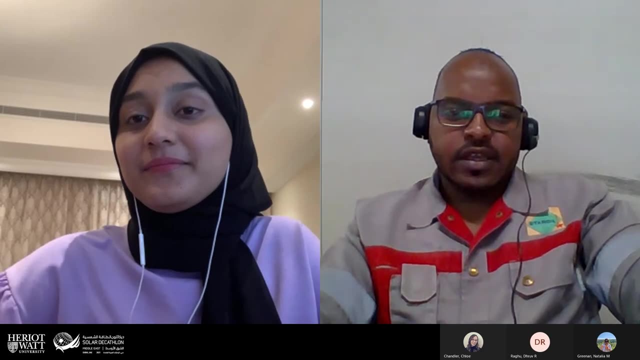 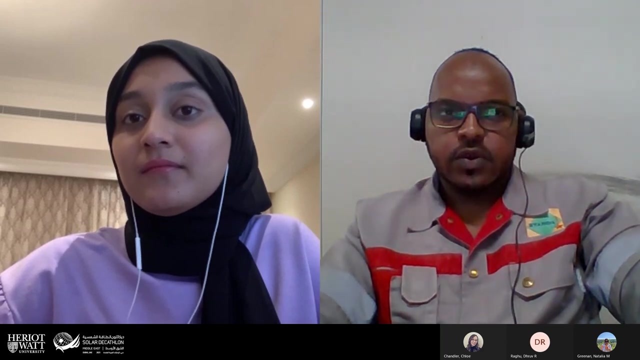 public, because sometimes public didn't have a a real information about the impact and about the environment. so they sometimes make some complaints and so you need to listen to them. you need- actually we, i need to- for to mention that the eia didn't conduct it by one. 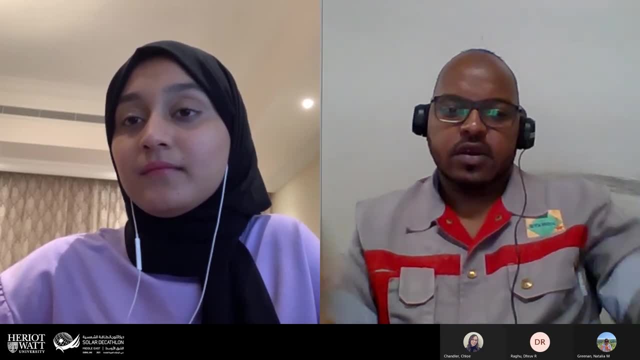 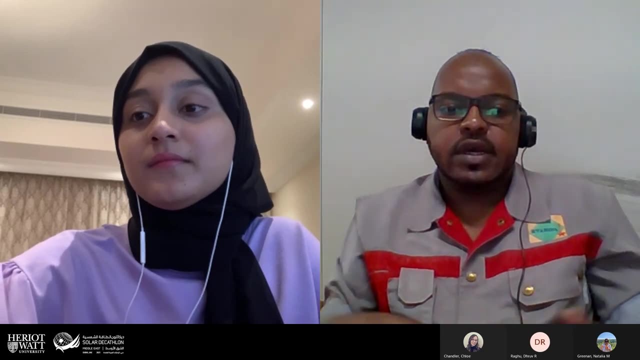 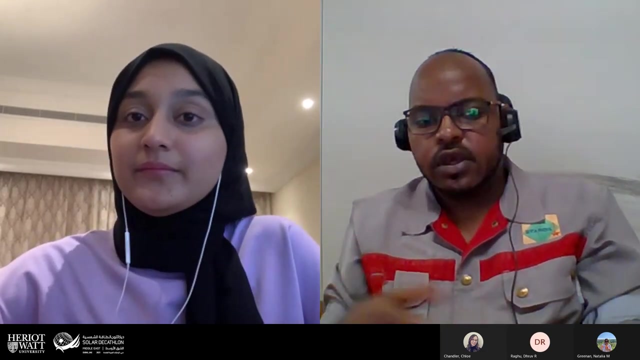 person could not conduct it by one disciplinary. it is multi-disciplinary uh approach, so need a multi-disciplinary teams. so usually there is some one uh expert in geology, one in the uh air and one in the fauna flora like this. so the team need to. 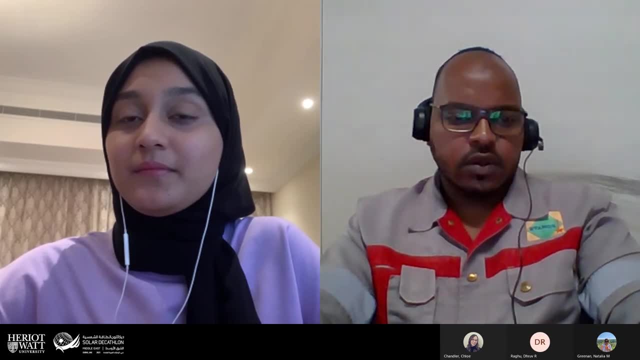 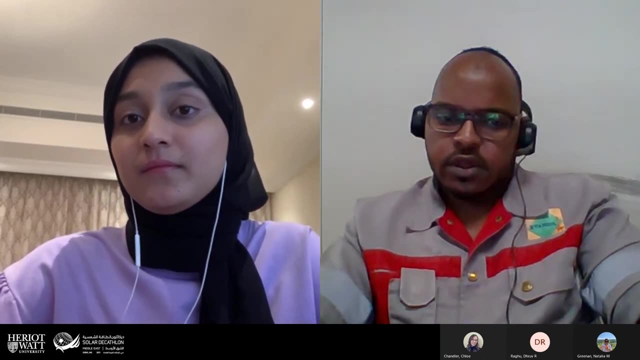 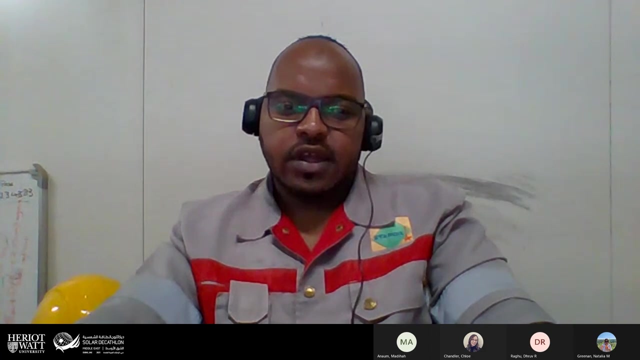 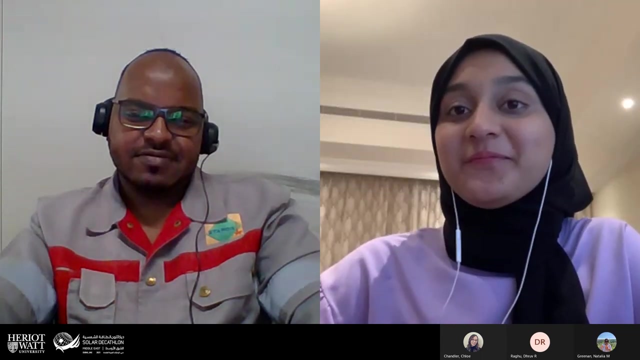 be very patient and listen, uh, carefully to the, to the people, and sometimes you, you, you get some very significant, important for a significant information from the local and from the public. so i do advise anybody to listen very carefully to the public and be patient. thank you for that. that was really helpful. uh, anyone else would like any?